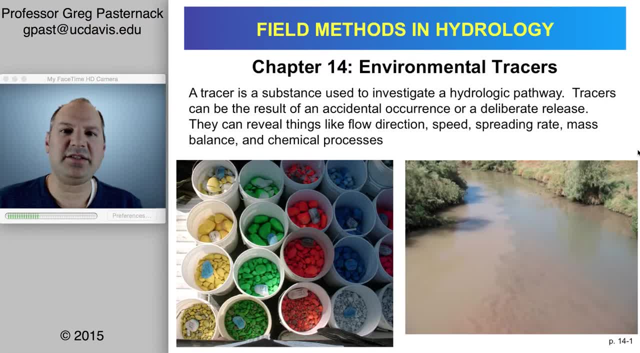 This is the video podcast for chapter 14 of Field Methods of Hydrology, and the topic is environmental tracers. This is part of the water quality section, for reasons that you'll see, hopefully, in a few minutes, why I've chosen to put this in here Now. why are we interested in? 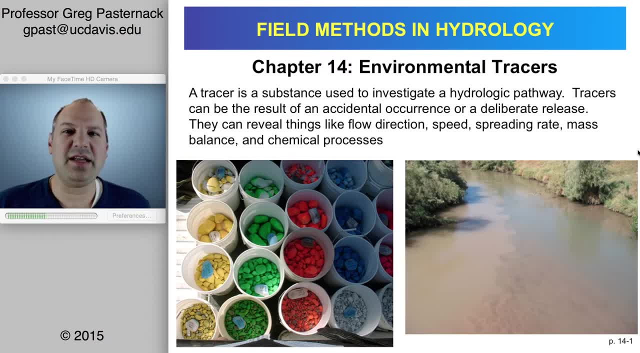 environmental tracers. Well, a tracer is a substance that's used to investigate a hydrologic pathway. Tracers can be the result of both accidental or deliberate releases, and they can reveal a lot of important things about what water is doing in terms of its flux, and even how much is being 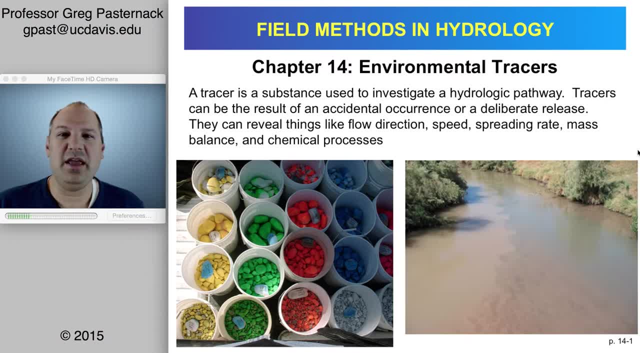 stored, but especially and most importantly, the mechanisms of how water is moving around. We can see speeds. you know, is something residing somewhere like residence times, like is it lasting there for years, hours, minutes? It helps us get at maximum speed and we can see how much water is being stored. So we can see how much water is. 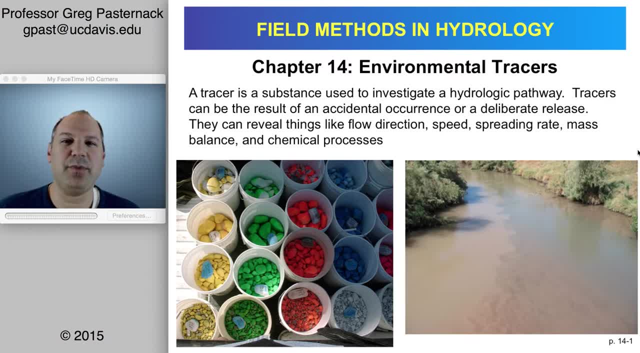 moving around. We can see how much water is being stored. So we can see how much water is being yielded and how much mass balance is, as well as chemical transformation. I want to read to you a little news article that had come out that shows about the importance of an example from accidental 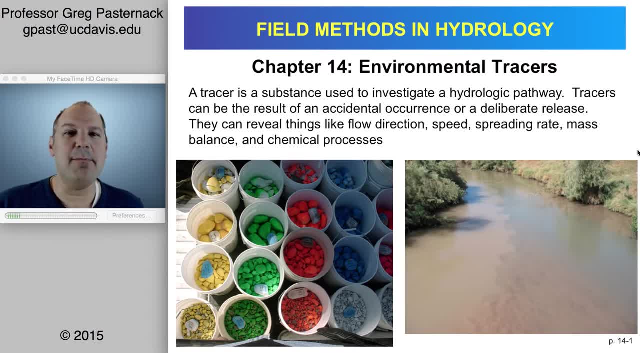 tracers, and accidental tracers are quite ubiquitous, so most of what this presentation is going to be about is drawing on accidental tracers, But I will also talk about deliberate tracers, which are really helpful if you're allowed to use them. OK, so the titus of this news, title of this news: 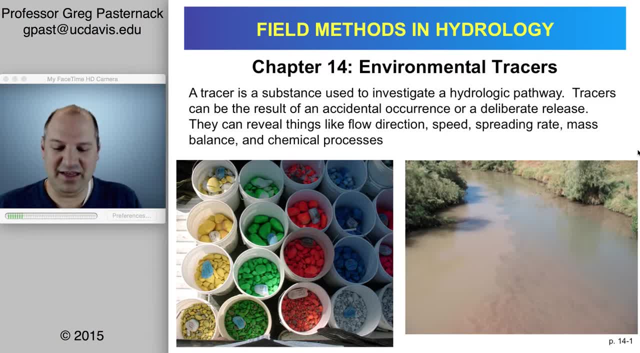 article was why oceanographers love plastic duckies. and let's see. um, i'm trying to see. okay, so these days, a huge number of plastic and rubber rubber items manufactured in asia are shipped in containers to markets and customers in north america. often the containers are stacked on the decks of ships. 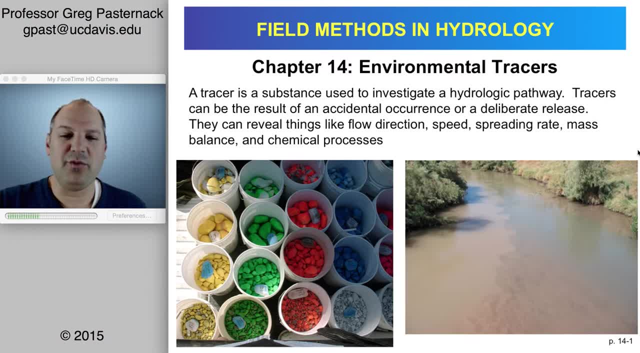 rather than stowed down in the hold. in rough weather in the north pacific, containers have been known to tear loose and be washed overboard. in 1990, a vessel container lost five containers overboard in a storm. four of them apparently tore open in the process, releasing 61,000 nike running. 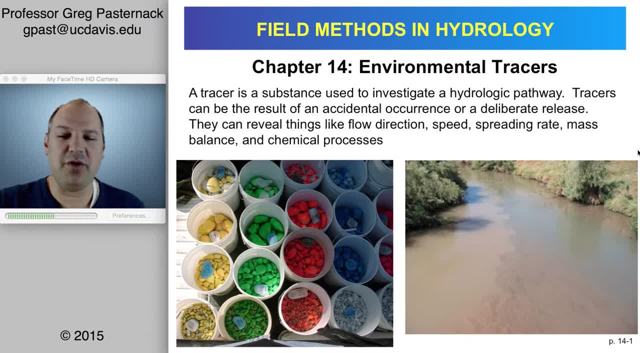 shoes into the pacific ocean. these shoes float and several months later hundreds of them began to wash ashore along the coast of north america, from alaska to oregon. beachcombers gathered them up and arranged them to be washed overboard in a storm. oceanographers were delighted. here was a unique chance to plot ocean currents and surface drift. 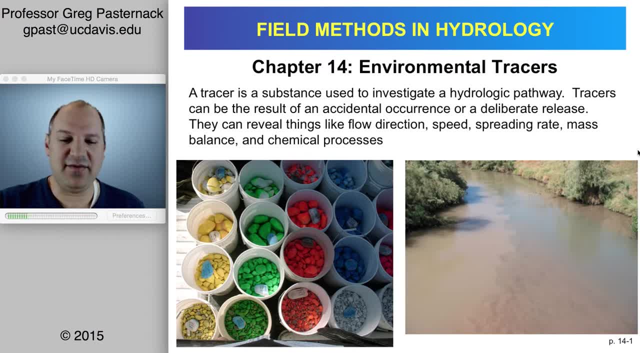 on a scale that could never have been done on a scientific budget. scientists tapped into the information network of beachcombers and the points of landfall of at least 1,600 nike shoes, and they were recorded exactly. this is about the same rate of recovery as those of the oceanographers who 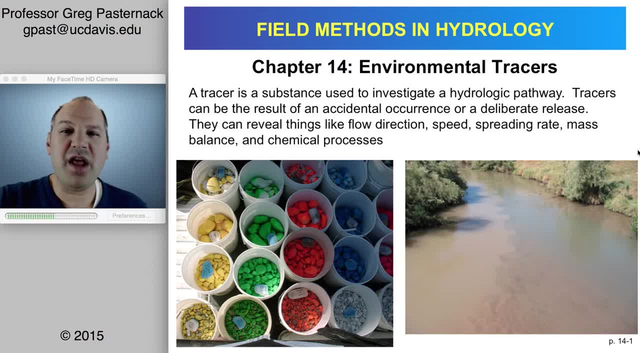 get from their drift bottles, but no oceanographer can afford to drop 61,280 drift bottles in one place at one time, by bottles. by the time the data were plotted, the drift of the north pacific was recorded in finer detail than ever. years later, far floating north, and nike shoes from the spill are still. 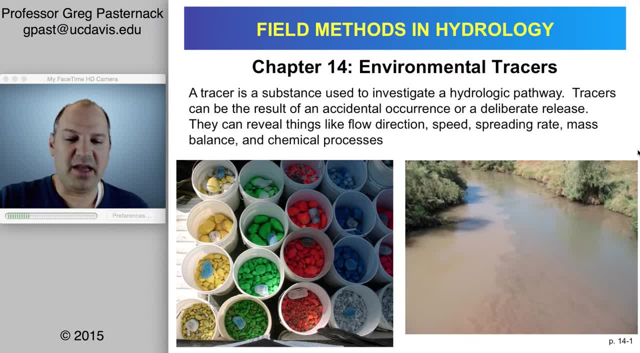 being recovered as far away as hawaii because the surviving floaters were turned southward into the main pacific clockwise circulation. it is with even greater delight that oceanographers learned the fate of 29 000 chinese plastic bath toys during their voyage from hong kong to tacoma. 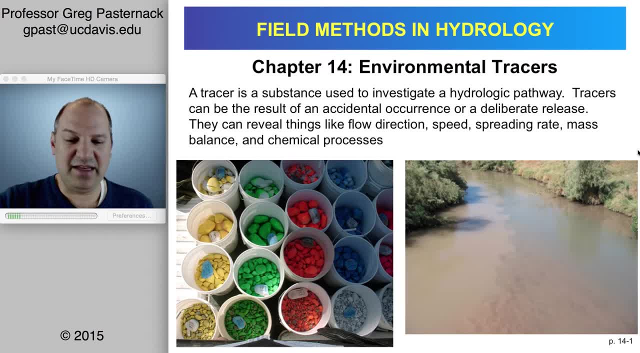 washington in a severe storm on january 10 1992, 12 containers were washed overboard. one of them tore open and thousands of blue plastic turtles, yellow plastic duckies, red plastic beavers and green plastic frogs began their great adventure. these animals are all competent swimmers. 10 months later, the first waves of plastic toys hit the. 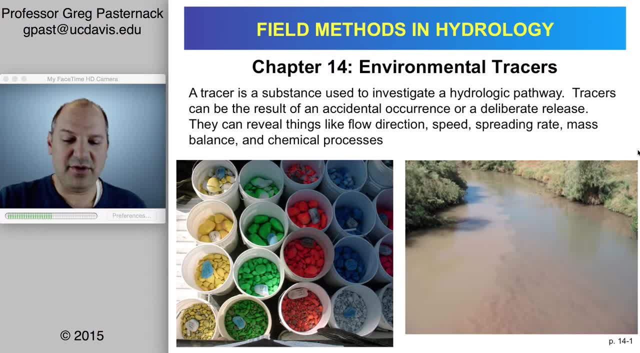 beaches of sitka. alaska. advertisements and newspapers and letters to lighthouse keepers brought in reports of landings, all of them on the alaskan coast. this time the higher floating plastic toys were more affected by the wind than the low floating nikes, and their main trajectory took them. 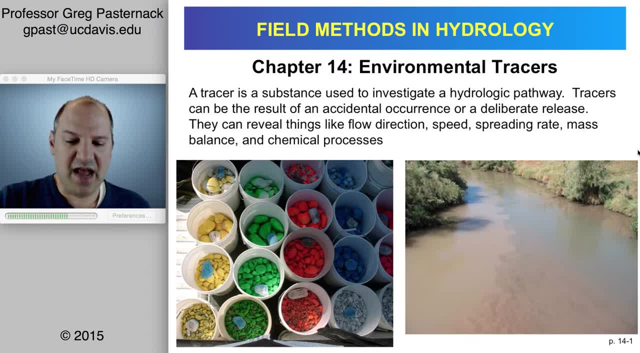 north. out of the gyre circulation, those that did not reach shore quickly were swept northeast and by the winter of 1993-94 the survivors would have been frozen into ice sea- ice in the bering sea. some may now be heading back into the north pacific. others may be on their way around the arctic ocean eastward along the north. 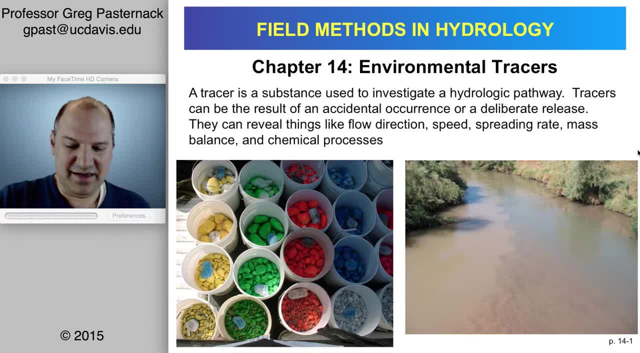 coast of siberia, heading for the north atlantic, and then in 1999, they don't make nikes or plastic ducks in europe, but they do make lego and they ship it out by sea. some five million pieces of lego that were dumped in the atlantic ocean are heading for beaches and they are now in the north. 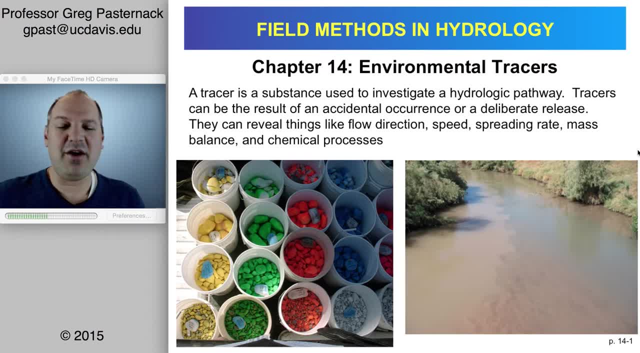 pacific, where beachcombers and oceanographers can find them. okay. so you know this is an example emphasizing oceans, but the same is true for hydrology, dealing with the terrestrial part of the world, that there are a lot of accidental spills that take place that we can make use of. 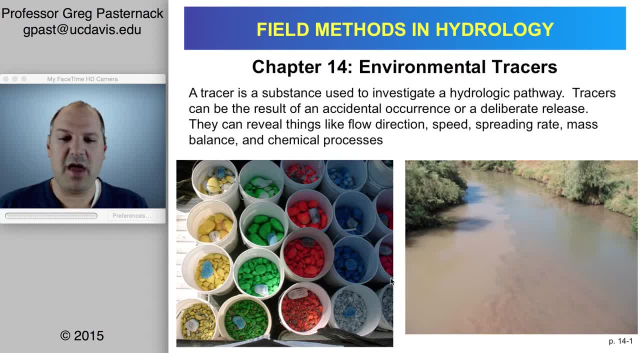 and just as some photos. on the left, here's a deliberate tracer painting gravels and cobbles to put them in a river to study sediment transport mechanisms, and on the right, here's an accidental spiller where two streams are coming together. one is receiving a lot of sediment from agricultural. 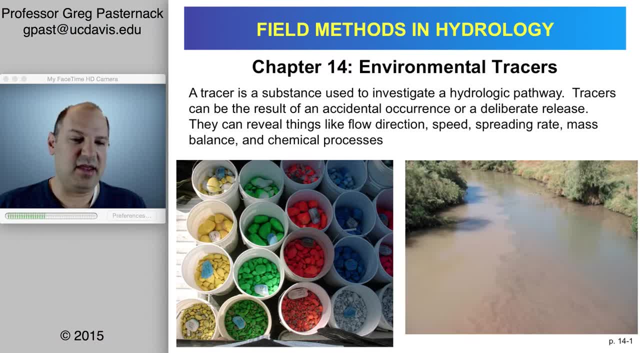 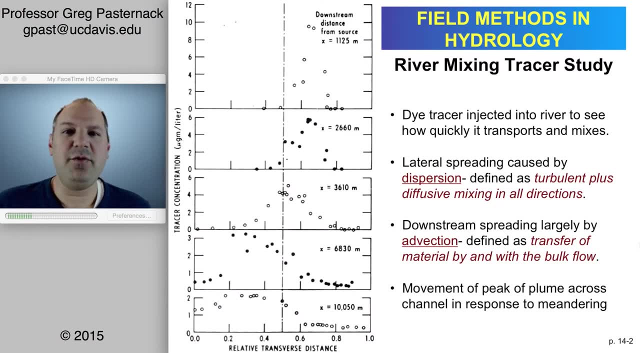 lands that are having furrow and sprinkler irrigation and then on the right, those irrigation methods are not being done on this particular day. let me show you a few examples of tracer studies used more scientifically- and these are relevant because you know this is a field- methods and 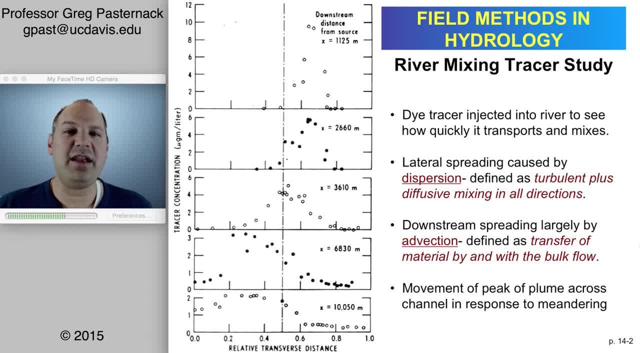 hydrology class. so i want you to have these ideas so that if you ever need to do a tracer experiment, then you have an idea of how to go about it. this is an example of a river mixing tracer study. in this case, a dye tracer was ejected into the river, so that's a deliberate tracer and they wanted 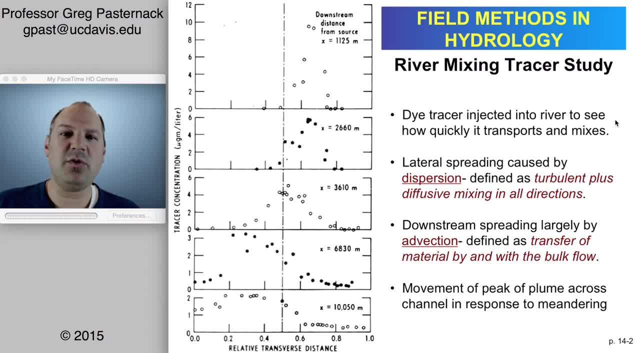 to see how quickly it transport and mixes. so this could be used for a model calibration and validation field study, because a lot of computer models have to do with contaminant transport or flow transport, and so it's a lot of work to do with contaminant transport and so it's a lot of. 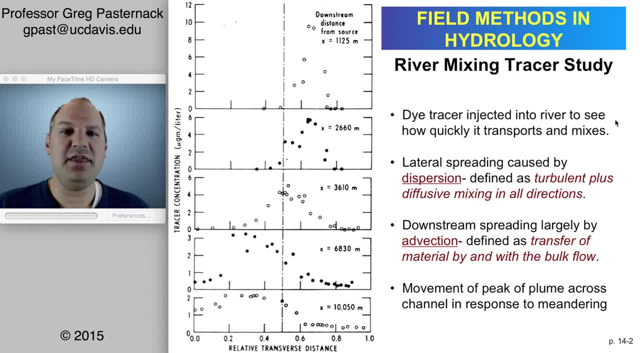 work to do with contaminant transport, and so it's a lot of work to do with contaminant transport and those cases. you need to get the mixing parameters that are used in the models, and this is what a mixing experiment like this would be used for. so here we have, what one, two, three, four, five graphs. 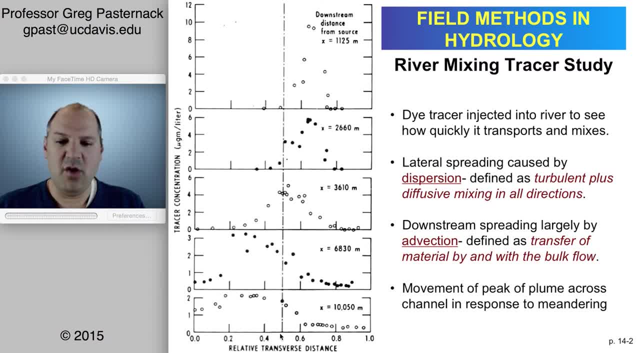 and the x-axis goes from zero to one, where the middle represents the middle of the river, the left represents the left side, with zero being the left bank. so, as you're going looking down the river, this would be river left and 1.0 would be the far river right. 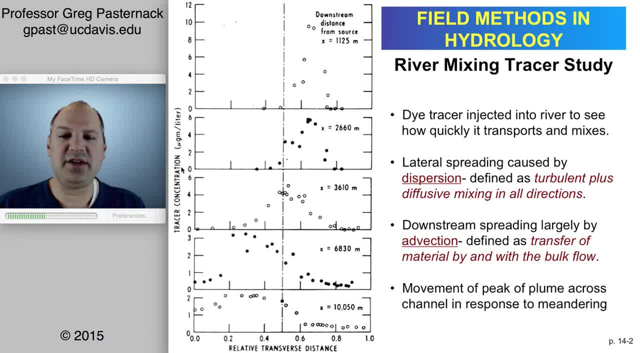 on the y-axis is the concentration of the tracer in micrograms per liter, and you can see that the concentration it's, it's uh, looks like it's well. the scaling is different and the range is different, so keep that in mind. and then, finally, the plots go from top to bottom, with distance from the source. 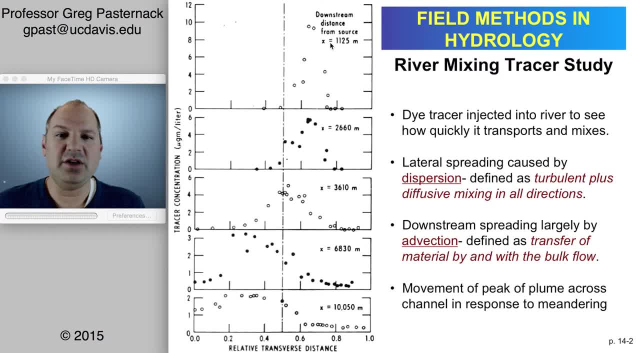 of the injection of the tracer. so we begin at 1.125 kilometers or 1125 meters, and then we go down in an even interval until we're past 10 000 kilometers down the river. there's a lot of things that you can see here. first, the spike is at its highest concentration, closest to the source, and that 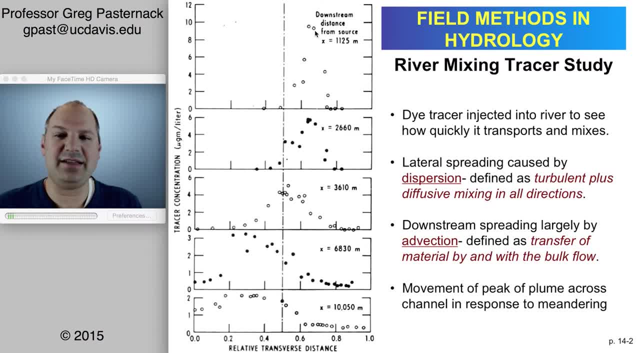 concentration peak drops from about, you know, nine to ten, all the way down to a little bit more than two by the time you get 10 kilometers down the river. second, we can see that there is spreading so um, if you look at the shape of this curve like, imagine this being like a. 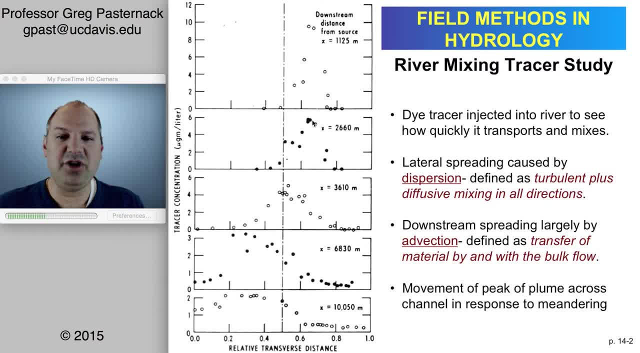 histogram. it's relatively spiky and as you go down, if you just stay centered on the peak, you can see that it's spreading out more and more and by the end it's the most spread out across the river. i mean, even you know up to, even you know, arguably, the 3.6 kilometers. it hasn't even spread. 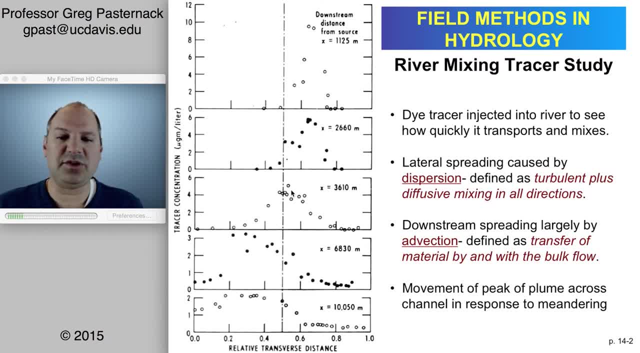 out all the way across the river. this kind of lateral spreading around the peak is called dispersion and it's defined as turbulent plus diffusive mixing in all directions. remember that flows and rivers are not laminar but they're turbulent because they're substantially deep and high enough velocity to create that kind of turbulent mixing. 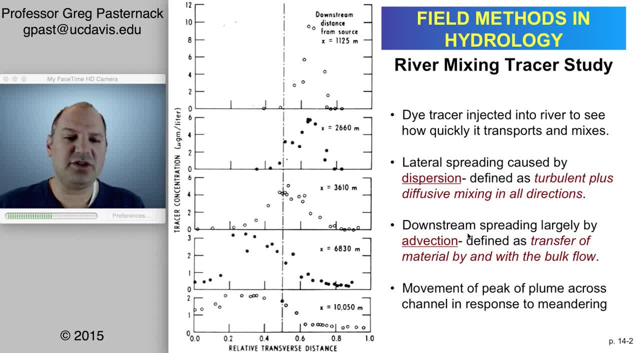 and so that causes a lot of spreading. there's also the downstream stream spreading. i mean, obviously the flow is carrying the contamination down the river and we just call that advection, defined as the transfer of the material by and with the bulk flow. you can also see that those streams are moving both from the right to right. so 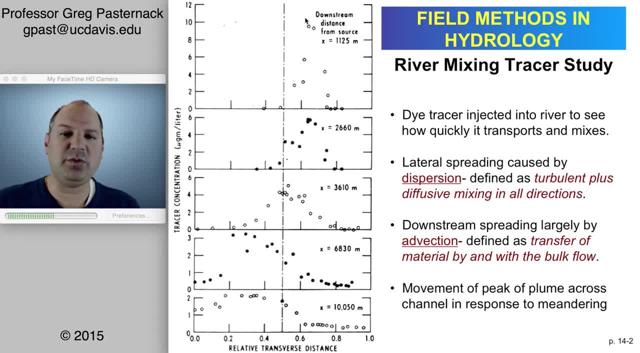 that's the flow. from the depth of the river you can see that most of the contaminant is just moving down the river, but some fraction of it is spreading laterally. and that happens in two ways. one, by just spreading around the peak, but then also the peak itself is shifting from right to 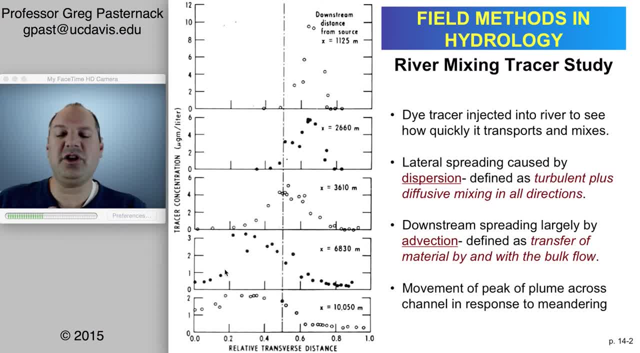 left and it's not shown here, but that's because the river is meandering and as the river meanders, then from one side to the other, the peak, you know that, like the bulk flow is going to be shifting the center of a riffle and to the other outer bank on the next meander bend. 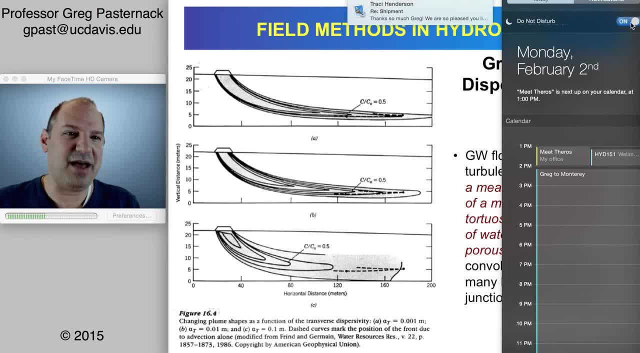 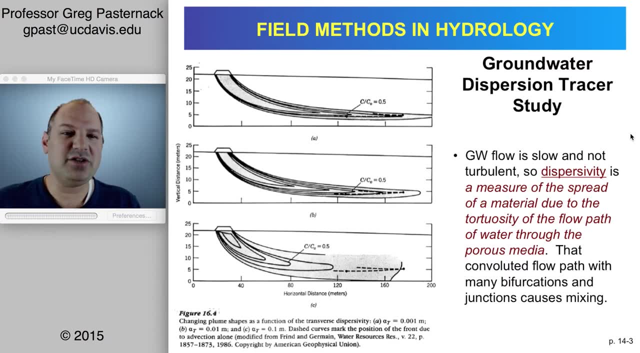 I don't want to see any notifications. Apologies for that. I always forget to turn that off. Okay, so the next thing: groundwater dispersion tracer study. So let's move from surface water to a groundwater example. In this case, we have a constant source of contamination. 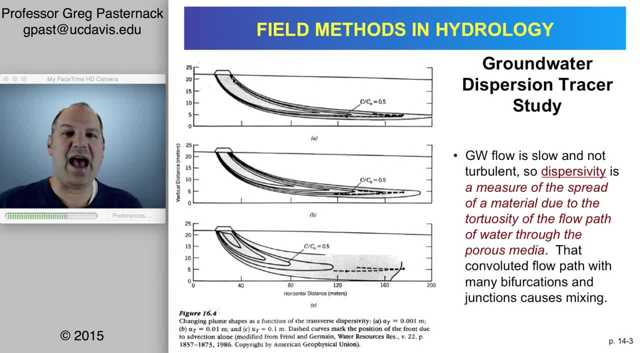 You could imagine something like a gas tank or a leach field, or it could be a septic tank, Something that is continuously putting out some form of contaminant, And then gravity is causing that aqueous contamination to move down into the ground. But then there's also the ambient. 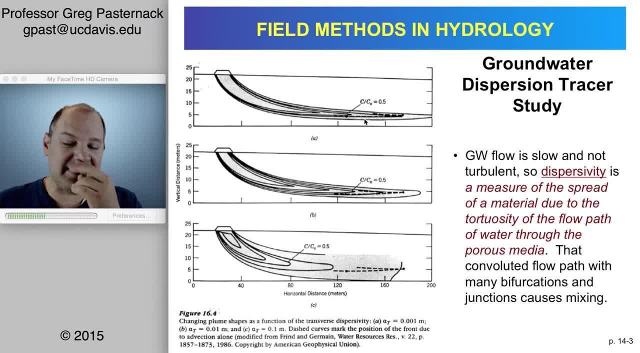 groundwater flow, which in this case is from left to right, And the x-axis here is horizontal distance, The y-axis is vertical distance, So we're anywhere from zero to 22 meters underground, And then the contours that are shown on this plot are the concentration of the contaminant. Now, actually, this is something I 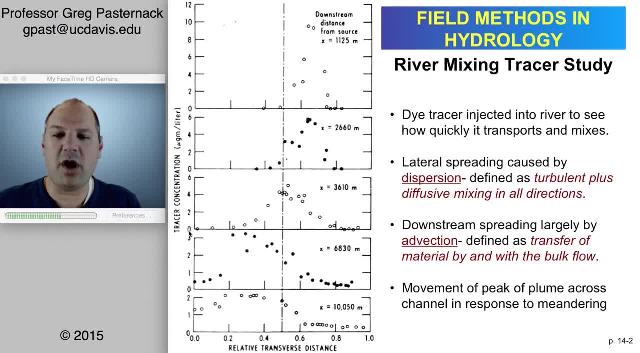 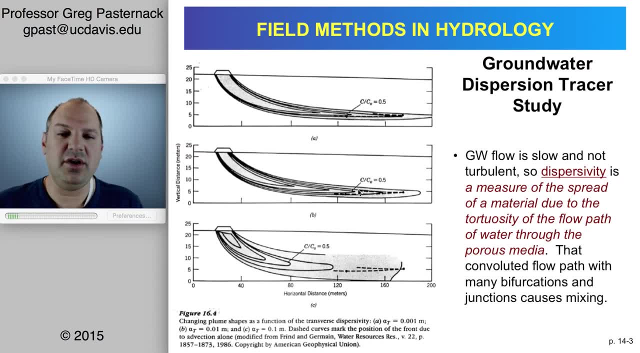 forgot. No, that wasn't there. Okay, in this one here we just had overall tracer contamination. Now we're going to change: Instead of reporting absolute value of concentration, we're going to divide the concentration at any point by, So that's given the symbol C, by C naught or C zero. What this is is the concentration. 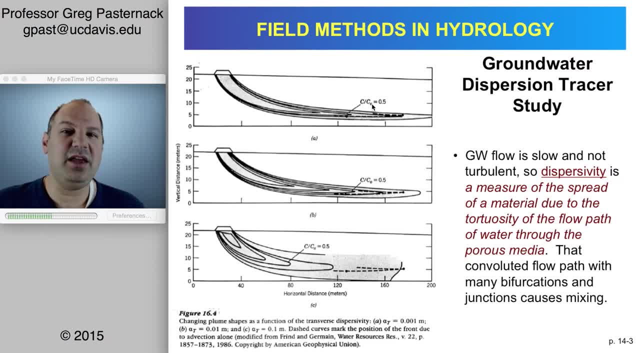 of the source. So typically, of course, there's no additional source, so the concentration can only go down, And so therefore C over C zero can only be lower than one. This is a very common non-dimensional way of looking at the spatial pattern or temporal sequence. 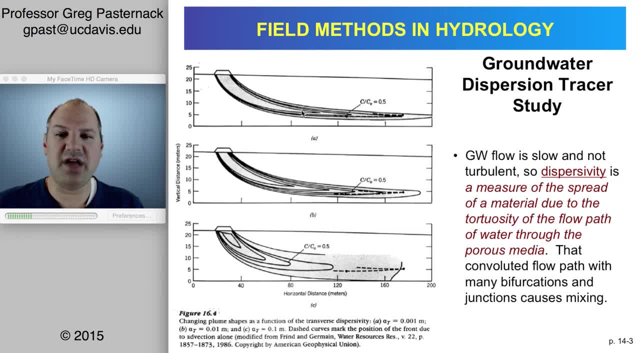 of concentration in a tracer. So we're going to do a little bit of a study And what you can see here are three different plots. These plots have different levels of transverse dispersivity. if you look at the figure caption, The dispersivity here, the top one, has a very small value of one millimeter. 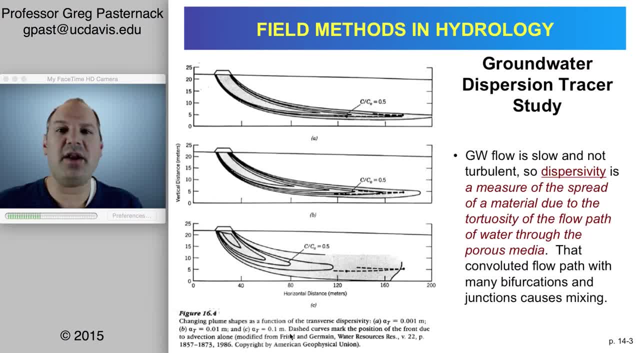 The second one has a value of one centimeter And the third one has a value of 10 centimeters. What this means is the larger the dispersivity, the more it can spread. And how does that spreading take place? Well, the ground is a porous media and flow is maybe going into the ground. 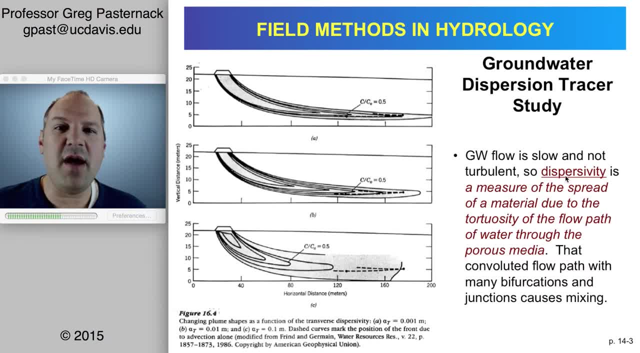 but then it's going to take a tortuous path because the flow has to move around the grains And as it does that, individual particles of pollution might make a left turn, a right turn, or go over the top, go under the bottom, And so they're going to be taking highly convoluted 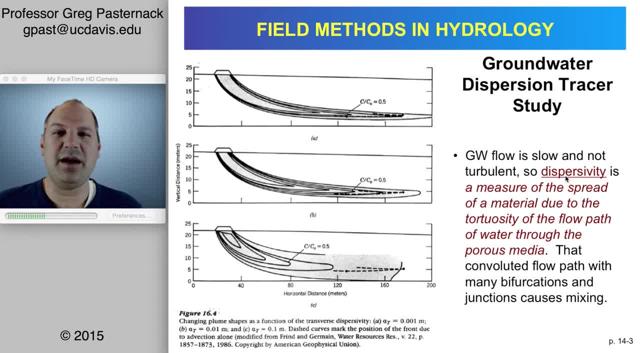 pathways. Ultimately, everything is going to get to some destination, And what we can guess is it's going to be a very slow והsep flow right, And this is because groundwater flows in this area more than normally down gradient moving. 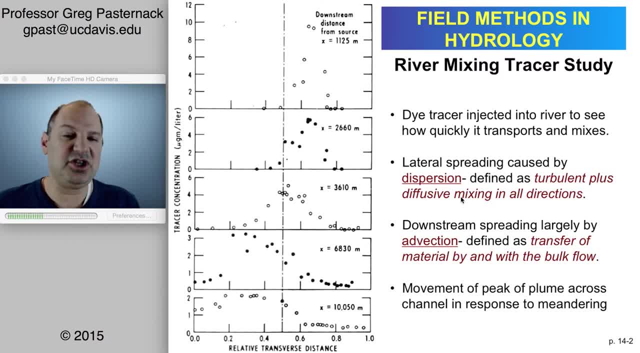 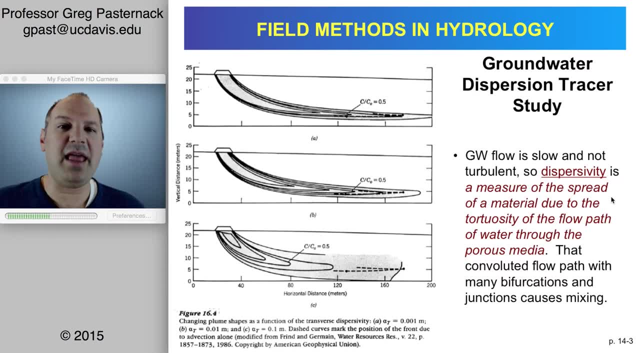 with the ambient flow, that advection. But the dispersivity here is different from the dispersion in the open water case because the open water case is just turbulent flow With groundwater flow. it's moving very slow and it may not be turbulent at all. It could. 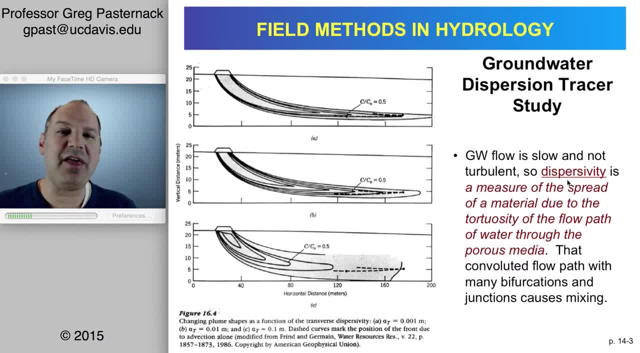 even be laminar. Most likely is because it's moving so slow itself, driven by the porous media, is causing that apparent mixing or spreading to take place. and you can see that with the highest dispersivity, the the size of the plume is the widest and as a result of that it's spreading more. 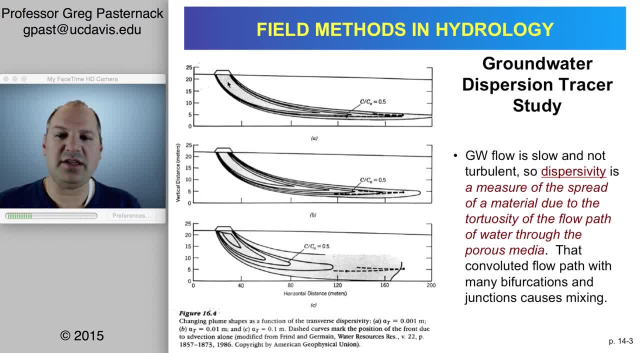 which lowers the concentration in other areas. so at the top plot, where we have low dispersivity, you have a very highly concentrated pathway with the C over C knot of 0.5 getting, you know, more than 120 meters downstream because it hasn't spread out. a variation on this theme is the situation that takes place when you 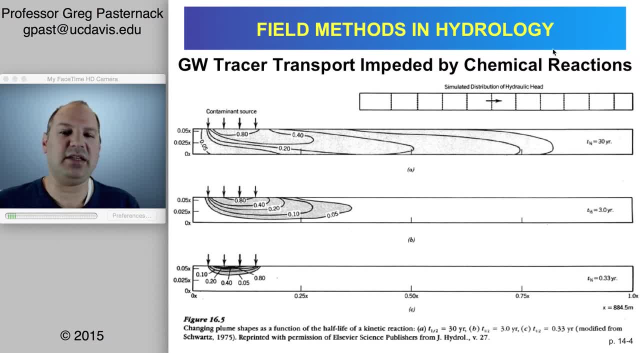 also have a chemical reaction that's taking place. so this is where, whatever the contaminant is or the tracer, it isn't just moving with the flow and spreading, it's also being removed through chemical transformation, and here we have kinetic reactions with either a 30 year. 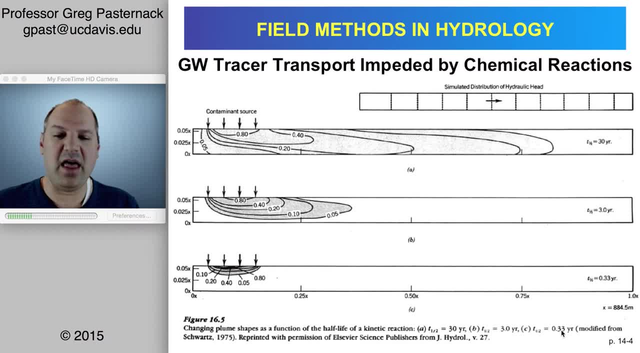 three-year or 0.33 year half-life, the the faster the chemical reactions are taking place, which is the bottom plot. so a half-life means half of that material has been eaten up or transformed in that time, while it's being transformed so quickly that it cannot spread very far before it's gone. and so, as a result, the 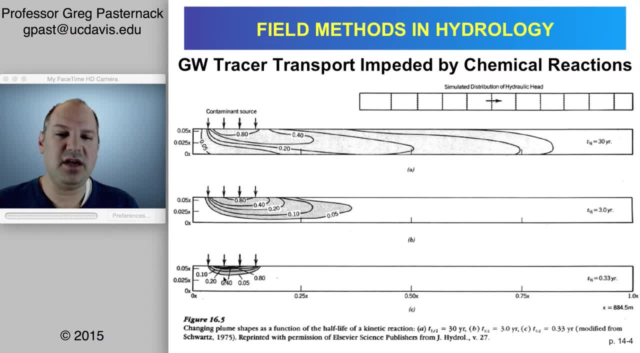 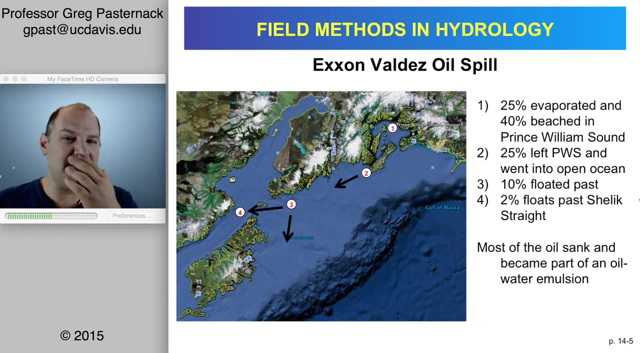 the contamination is highly concentrated near the source. at the other end of the spectrum. you have a very long period of time before half the material has been transformed. then you can have a lot of spreading taking place. as just one last example related to chemical transformation, we have the case of the terrible Exxon Valdez oil spill in the 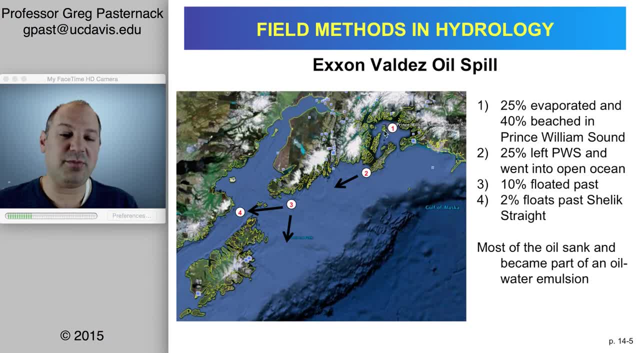 Gulf of Alaska. remember that? or that took place in Prince William Sound and what happened is here at Prince William Sound, where the number one is located on the map. it's pretty interesting of that material that spilled twenty-five years ago, Twenty-five percent of it evaporated and forty-seven percent of it beached. of what 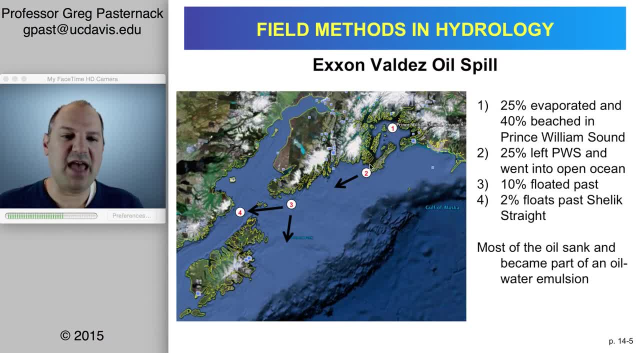 went out twenty-five percent. well, twenty-five percent went out, basically into the open ocean, but as it continued to move, more things are happening. the oil sank and it became part of an oil water, water immersion. so as the currents continued, by the time you get to point three there was only ten percent left, and by the time you get to this other coastal 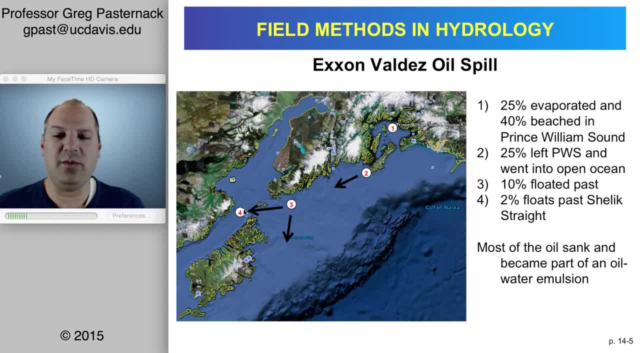 area by point four, then only two percent was into that straight. so there is really devastating consequences in Prince William Sound. but it's just really interesting to see that we have these transformations that are taking place of evaporation, sinking and emulsification that cause this contaminant to become less available, to cause environmental 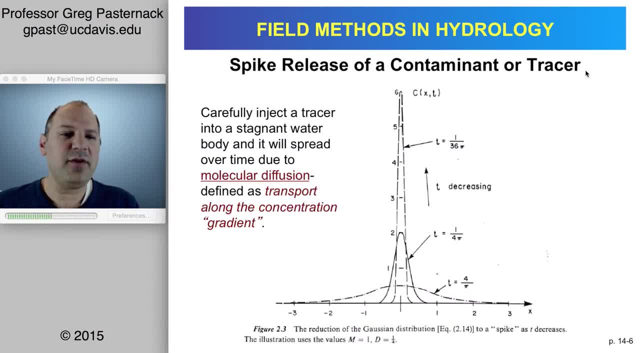 impacts. So let's turn from those fairly practical examples and definitions to just some more fundamental understanding of what's happening with the tracer. One kind of release of a tracer is called a spike release. so you put it in, it's there and then it diminishes. and if we just stay centered on a spot with no ambient flow, you 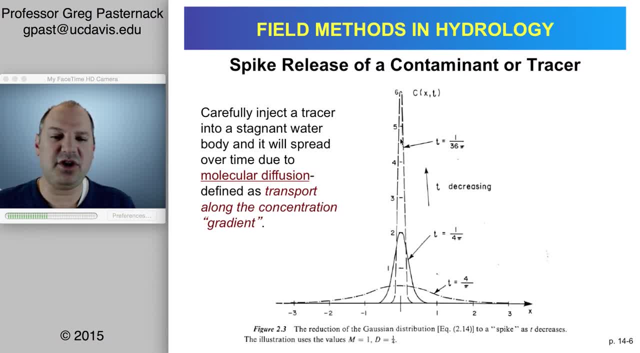 would expect that that high spike of concentration is going to be decreasing from time one to time two to time three. so through time it's going down And then, as it goes down, it's spreading laterally around that center. This is a case where this is primarily just molecular diffusion, so it's equally spreading. 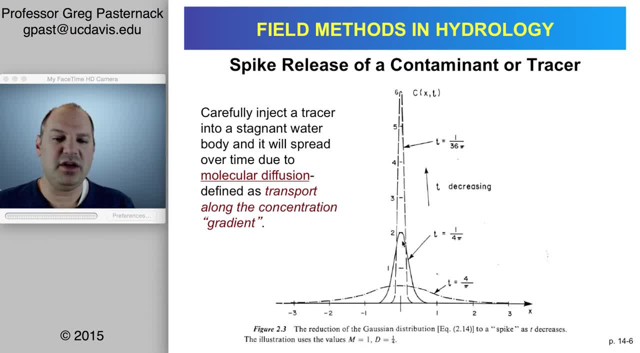 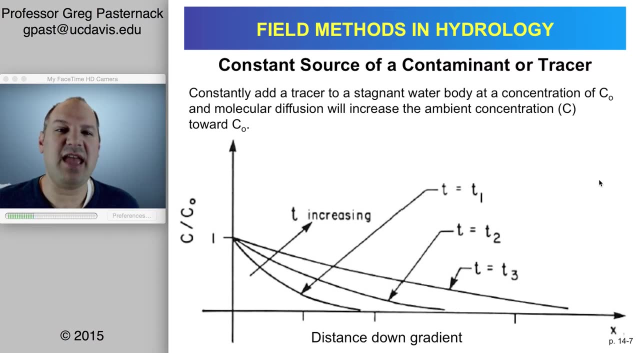 in all directions. this is just a two dimensional spreading example. well, I mean, it's one dimensional- left and right I guess, but anyway the concentration, and it's spreading across this line. Another example is a constant source of a contaminant or tracer And here, at this location, zero, we're holding the concentration of the contaminant or tracer. 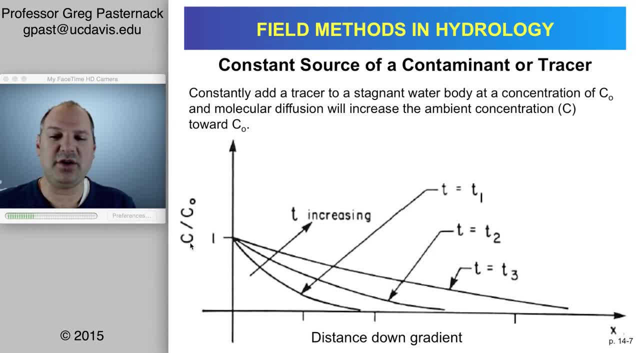 constant at a value of one, so the concentration equals the injection level, and then it's decreasing as you move downstream from there. but over time, because we're holding this constant, the concentration is increasing more and more, so it's spreading both in the downstream direction and the concentration is increasing downstream. 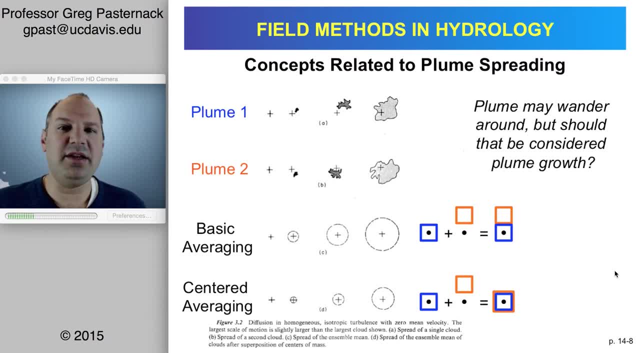 One of the challenges that comes up in dealing with tracers is deciding how to quantify the data. So imagine that we have a plume of contamination. The plus shows the location where it was in the first time. it gets released basically as a spike. 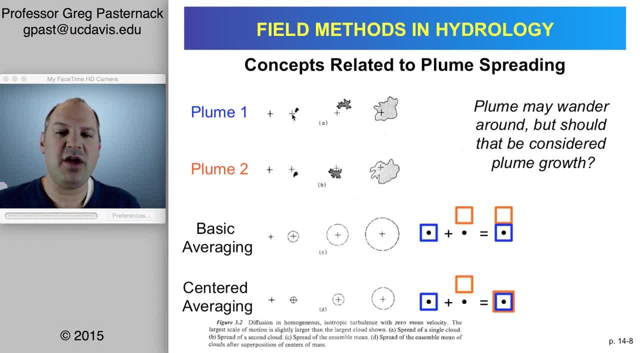 Now we're going to go to time two and here's the center and you see this very high concentration. this little dark blob, It's now Advected downstream somewhere or it's advected somewhere off the plus. At time three it's advected and spread, so the concentration is a little bit lower and 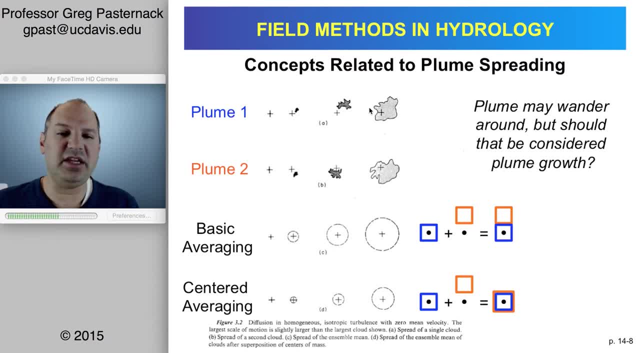 we see it's more spread out. At time four, it's primarily spread, the concentration is lower and it's back located off the peak. Now let's do another tracer experiment and with another plume and you have another example, or what we call a realization, of this contaminant transport. 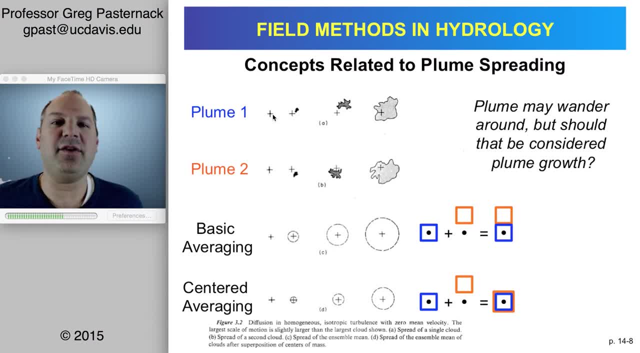 So the question becomes: if you want to characterize the average condition of this tracer study, how would you put together the data from plume one and plume two? There's two ways to do that, depending on what you want. The first is to use basic averaging which just says for any- you know any- pixel or square. 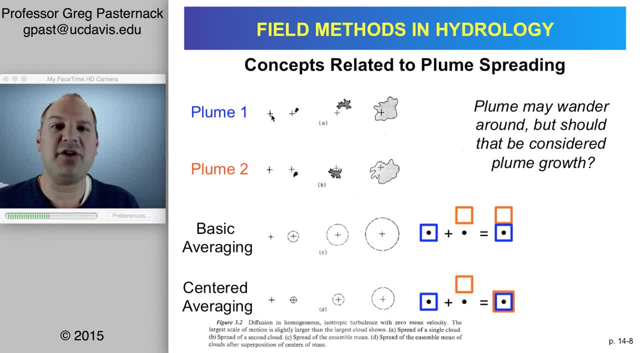 or whatever any location relative to the center at the plus. what is the concentration in plume one and plume two? And I'll take the average of that at each time interval. when you do that, you're primarily going to see the spreading that takes place regardless of where the center of the plume. 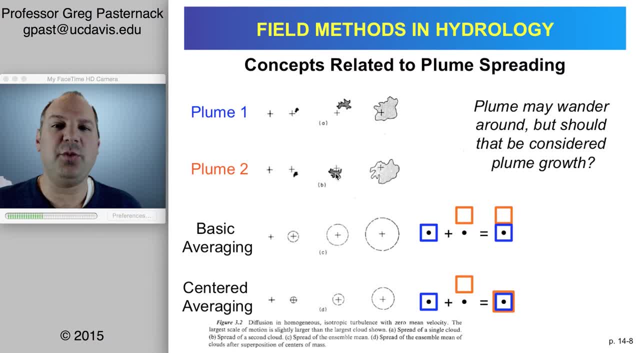 is located. So both advection and dispersion would be represented by basic averaging. So, for example, if we look at this, these blue and orange squares that I've shown in the imagine a case where, in time two- Assume, I'm sorry- time one, plume one- we have a centered plume, and then time two, we have an effective 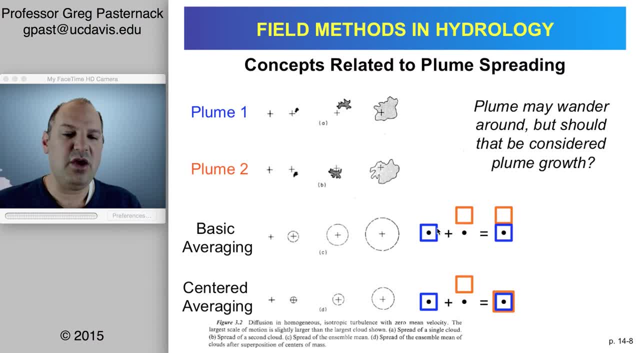 plume, but they both are spread to the same degree. when you average those together, the size of the plume would be double and you wouldn't be seeing the fact that it's staying as a coherent body with a tight distribution around the center. instead, you would see the 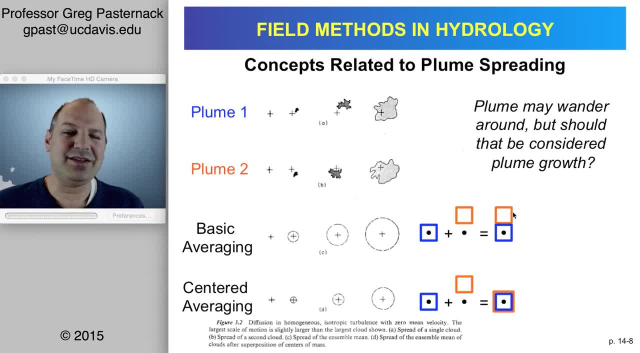 overall mix of the orange plus blue. So this could be a little confusing, But the idea is: you're just at any location. It's the average of what happens in the two plumes, without being mindful of the nature of spreading, And so the outcome is that because the orange is up here and the blue is down here, then 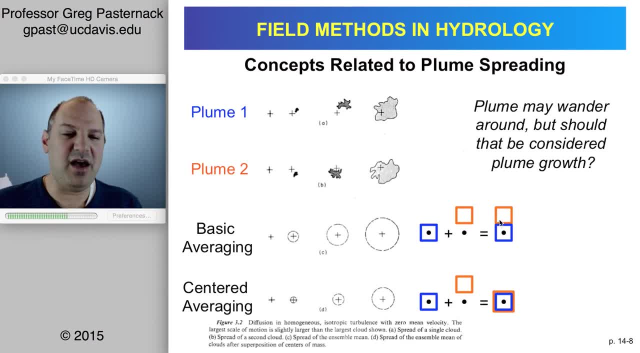 when you average those two together, half the concentration is above and half is below, And so it looks like one big plume with half the concentration spread everywhere. Another way to go is to stay centered on the plume, move with it like every time, step adjust. 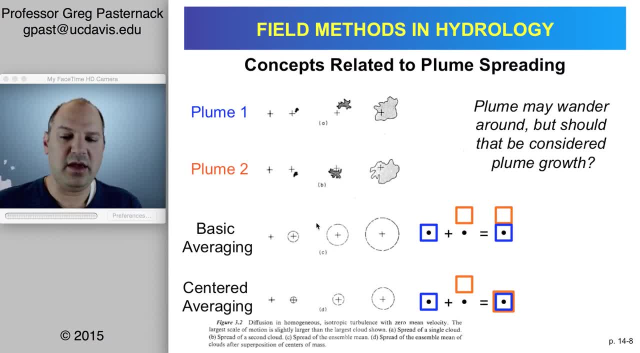 the plus to be located at the center. This is called centered averaging. in this scenario, in the, in the end you have the same outcome, where each plume has maintained the same shape and size and concentration, But of course the orange is shifted. But now we're going to move the center into the location where the plume is and therefore 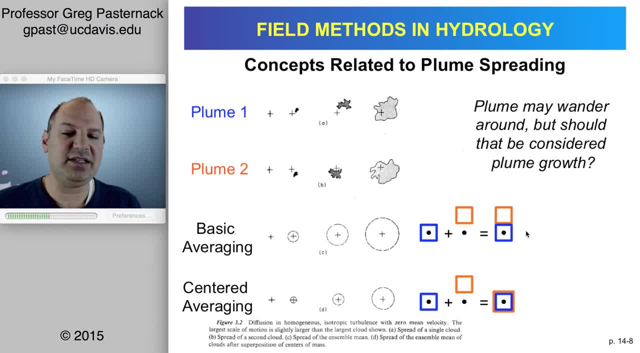 the size of the plume will be half the size of the basic averaging. Now, as I'm talking, this is feeling somewhat esoteric, But it's actually really, really important, because what this has to do with is like if contamination is taking place, and especially if you're doing a tracer study, the actual 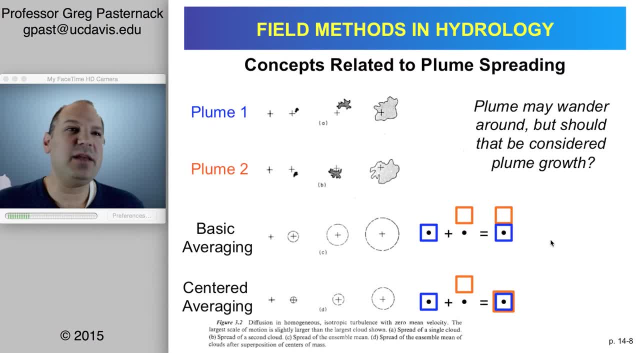 path that a contaminant is going to take. it depends on something that's highly variable, like just this dispersivity concept. especially if you're in a porous media Or if you're in a surface flow, it could be a result of the discharge and how turbulence. 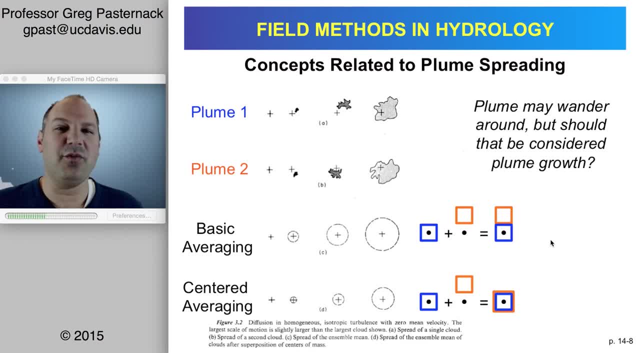 the area of inundation and pathways change depending on the roughness that's in the river at that flow. So what that means is like: do we just want to know in general where it goes, which would be the basic averaging, or do you want to see how the plume is moving and spreading? 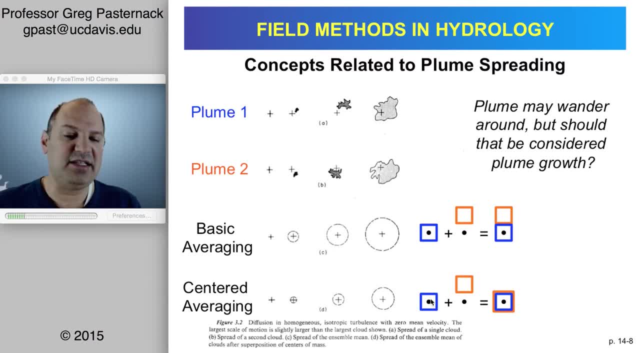 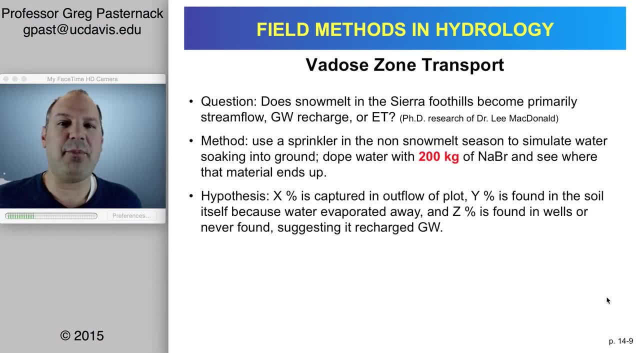 I don't care where it is. I'm going to follow that plume and see what the nature of spreading is, without worrying about the advection. Let me show you another example of a use of tracer That isn't about transport so much as more of like a mass balance. 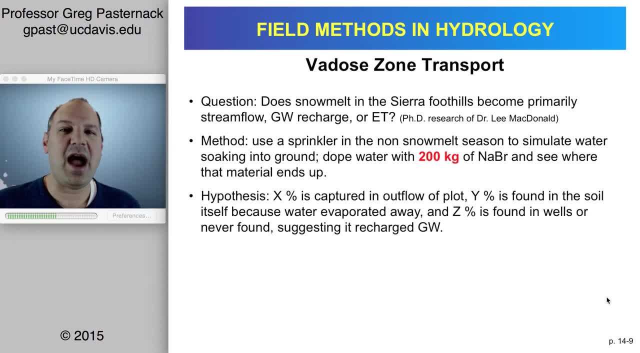 I'm calling this vadozone transport, but it's really also a hydrologic balance, because we're going to use a mass balance approach to figure out where stuff went. So let's ask the question: does snow melt in the Sierra? foothills become primarily stream. 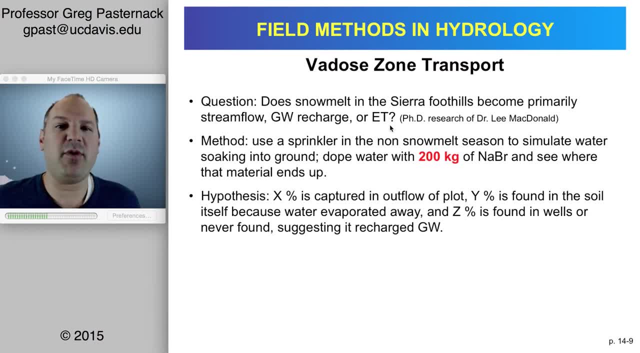 flow, ground water recharge or evapotranspiration. This has always been important, But the reason why it's important has changed. Historically, it was important for understanding supply of water, whereas more recently people might be more interested in environmental consequences of water conditions. 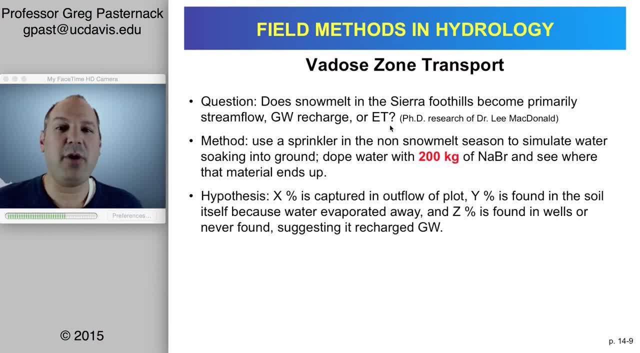 We're also seeing, with drought and climatic change, that people are once again also concerned about water supply, And this is work that was done as part of the PhD by Dr Lee McDonald, who went on to become a professor at Colorado State University And really did fantastic research on cumulative impacts: impacts of land use on watershed scale. 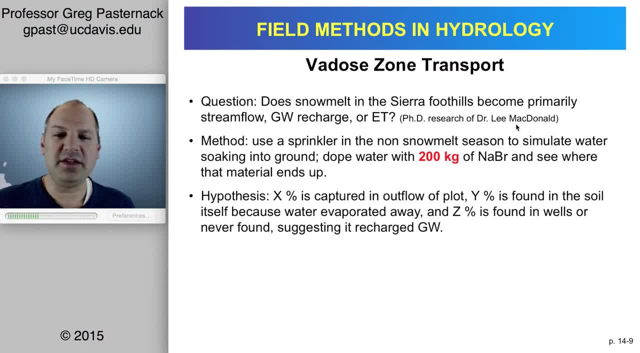 water and sediment movement. So in this PhD research the approach was to use: so, okay, we're interested in snow melt, but the first thing is we're not going to study snow melt because we want a controlled experiment. We're going to pretend that the water is on the ground and melting, you know, and moving. 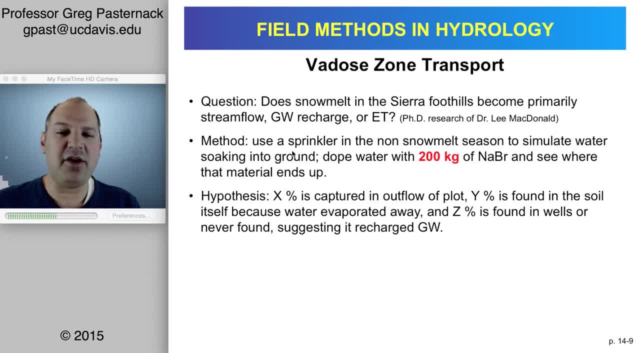 like as if it was snow melt. So in the spring, take out a sprinkler And simulate water soaking into the ground and then see what happens to that. In this case, the water wasn't just water, but there was a deliberate tracer added, which was 200 kilograms of sodium bromide. 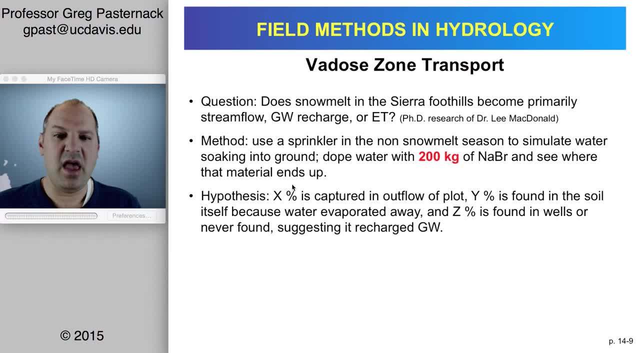 And then he went to see where that material ended up. We're going to make a hypothesis: Some percent of it is going to be captured in the outflow. and here what I mean plot, I mean like an area of the ground Over which this sprinkling is done. and remember, I think I talked about sprinklers a little. 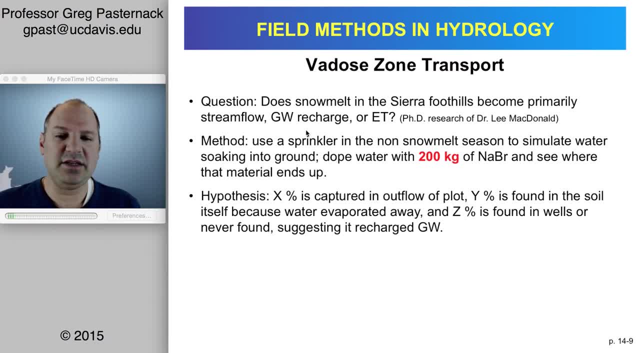 bit in the precipitation video podcast. So what percent of it is just captured? what, okay? what comes out of the plot and moves down the hill slope? What percent of it is captured in the soil itself, because the water evaporated away, And then what amount of it is found in wells, indicating that it went down into deeper groundwater. 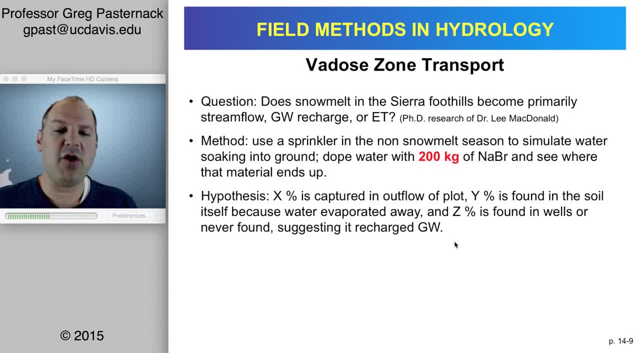 or is just never found at all. Okay, So I want you to pause for a minute and think about this before I show you the answer. If you sprinkle water onto the ground in the springtime, what fraction of it do you expect to run off as opposed to be stored? 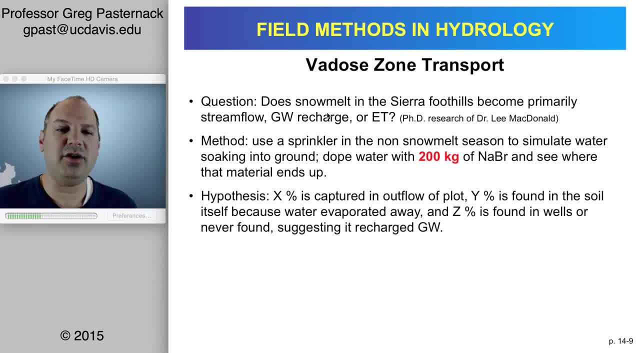 And this basically would tell us something about the fate of snow melt during during the spring. So hopefully you've paused and the answer is that out of 200 kilograms, only 20 kilograms were recovered after two years of monitoring the outflow from the plot. 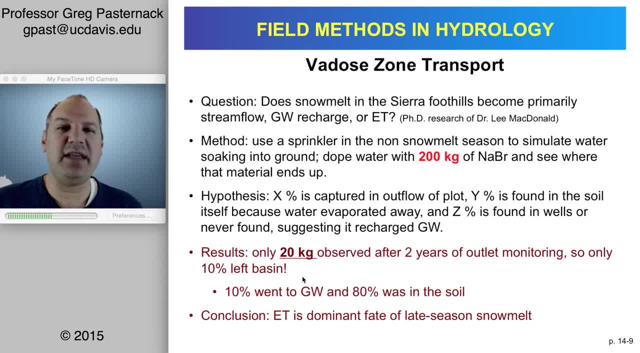 That means that only 10 percent of the tracer left the basin and by mass balance, that means only 10 percent of the water left the base and as surface outflow. Ten percent of it was found to have gone to groundwater, but 80 percent of it was found 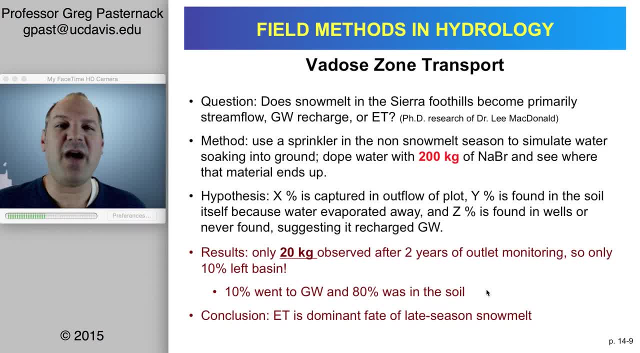 in the soil. Indeed, he was able to dig into the soil and find all of the salts that had precipitated there, which is a pretty staggering amount. I mean, in a way, this is fairly consistent with what we expect from surface water hydrology, in that, typically, runoff is 15 to 25 percent of rainfall. 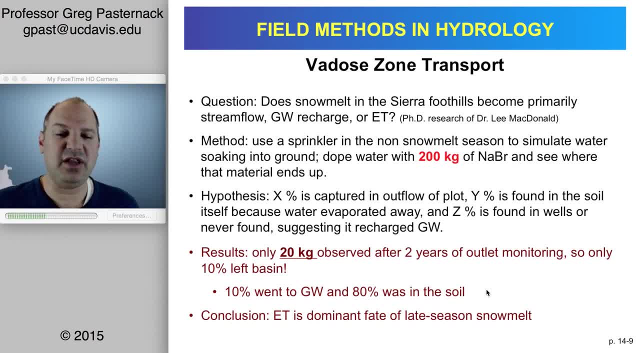 However, if the ground is already relatively dry, it could be substantially less, and that was found here. So the conclusion was that evapotranspiration is the dominant fate of late season snow melt. Okay, Now that I've shown a range of examples and applications of tracer evapotranspiration, 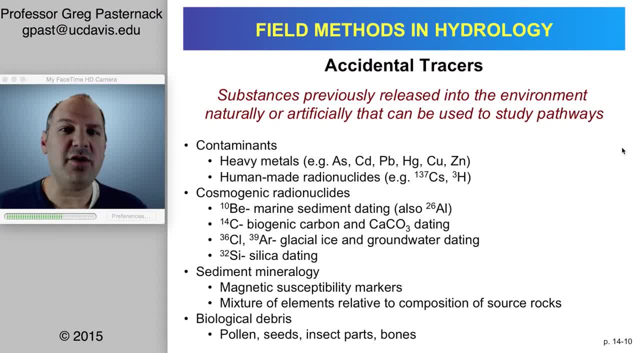 I'm hoping you have a good idea of the value of environmental tracers for hydrology. You've seen us use them to look at how water spreads in the surface water and groundwater, how it relates to the spreading of contaminant plumes, involvement of chemical reactions. 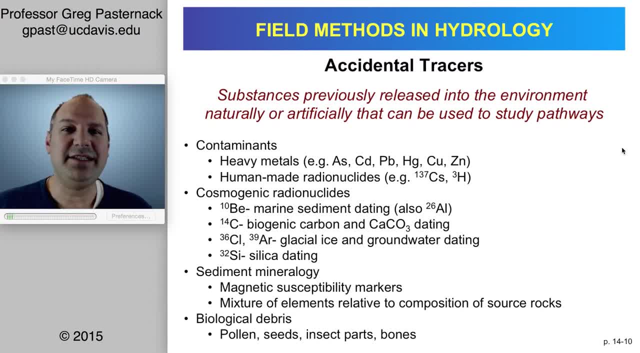 everything, including rubber duckies. So what I want to do now is dig deeper into the available methods you have, particularly in the field of environmental research. I want to show you a few examples of these methods. One is the use of accidental tracers, but also somewhat for deliberate tracers. 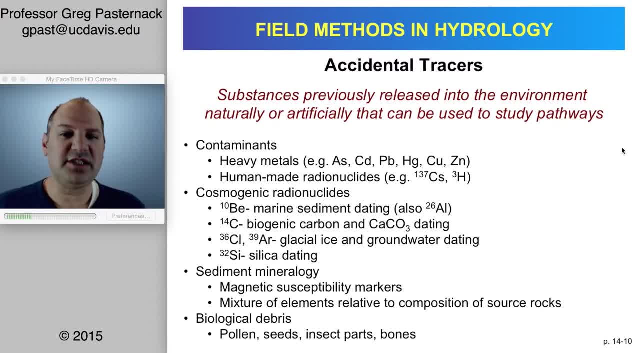 So accidental tracers- to give a formal definition- are substances previously released into the environment, naturally or artificially, that can be used to study pathways. Naturally you're going to see things like isotopes or heavy metals, and artificially you can also have those in other constituents. but then there's a variety of other things. 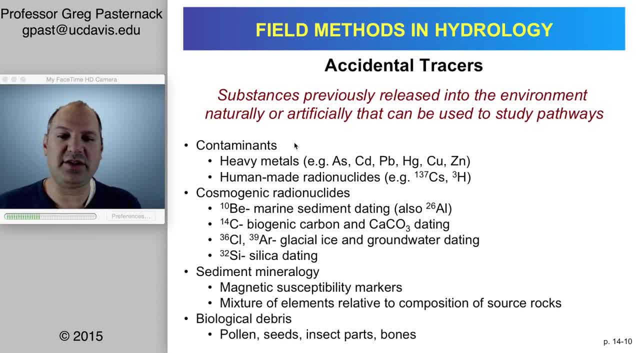 So contaminants, So contaminants. There's a huge class of tracers. Humans have put massive quantities of pollution into the world, and those contaminants typically have been done using heavy metals. Mercury is a very commonly used one: Lead, cadmium, arsenic. 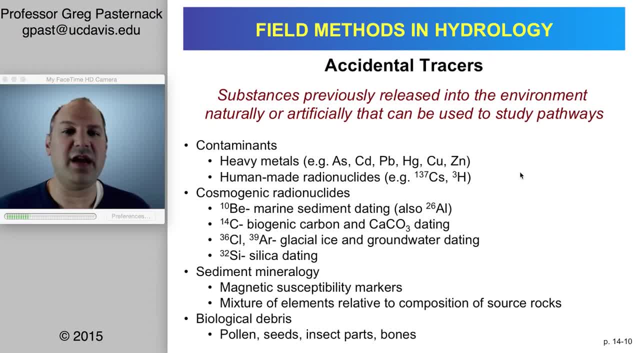 Just look to see if there's any waste water treatment plants or any other industrial facilities or mining operations, Things that are using and releasing contaminants Or, you know, as a result of, say, mining, making things available, tailings and so forth that would have that present. 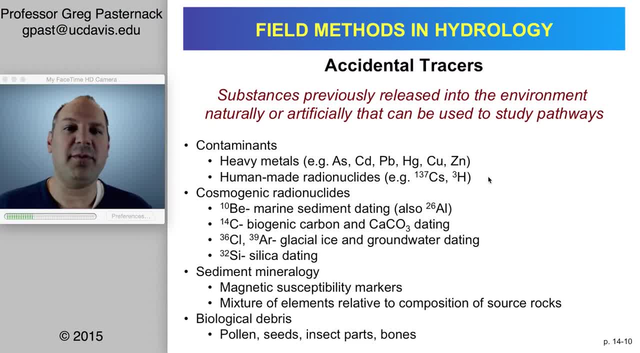 Human-made radionuclides, particularly from atmospheric bomb testing releases of cesium-137, but also tritium. There could also be organic compounds that are used, although they're not here, but things like TCE would be another example potentially. 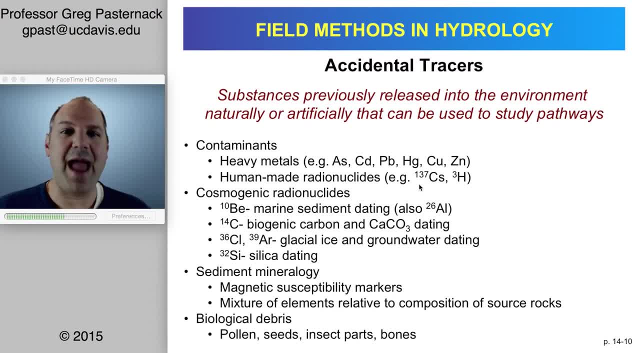 Although those tend to be highly reactive. so that is a little bit different. Cosmogenic radionuclides: these are a result, like being produced from interaction of particles from the sun interacting with the earth, And ones that we see here: beryllium-10,, carbon-14, and these others that are used 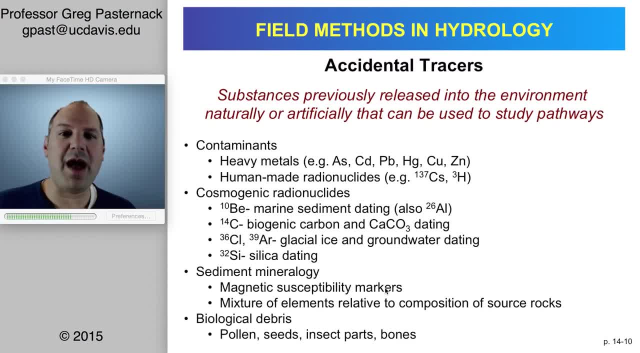 And I'll show you more about that in a moment: Sediment mineralogy. So just taking advantage of the fact that The ground, you know the subsurface, is composed of different constituents And, as a result of weathering or erosion processes, they can be released from their source to the sink. 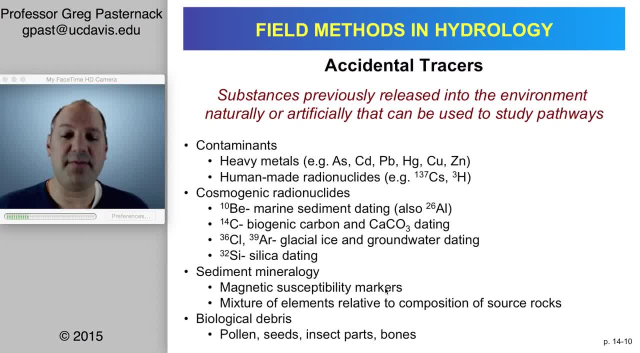 And so that can help you reconstruct source and pathways. And then biological debris, which can be indicators of the integrity of a biological system that are recorded through time in sediments, And I'll be giving more information about all of these, But this just puts everything in one place. 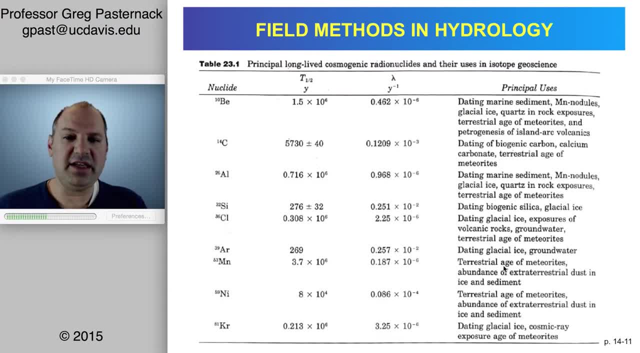 Okay, Here's a list of some long-lived cosmogenic radionuclides, and they're used in isotope geoscience. Now there are many more than these that are used in agricultural and environmental applications in hydrology, But this just shows some of them. 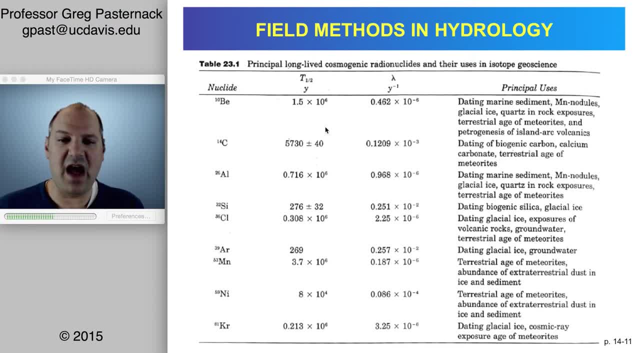 The half-life here in years. these are generally on the longer side, but not all of them. So, of course, carbon-14. Radiocarbon dating. This has been the big workhorse for studying human-relevant time periods in the last you know, really 35,000 to 60,000 years. 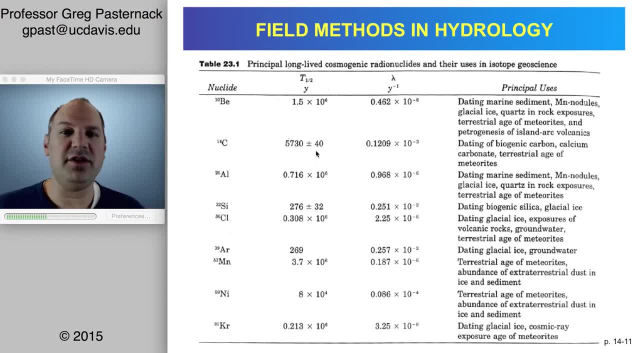 It has a half-life of 5,730 years, So it's not going to be so useful. things that are really young. Some of these others are quite long, Some of them are short And you can read on the right. you know what their different uses are for. 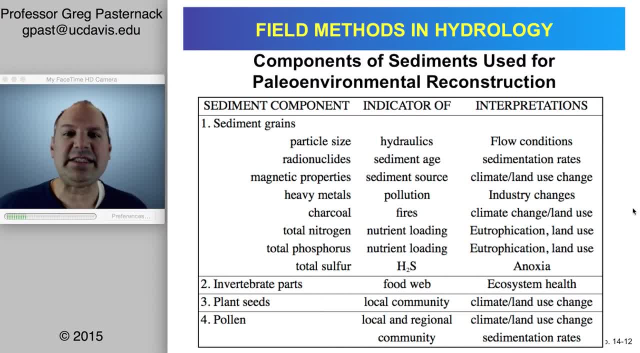 If we look at the sediment, so sediment is a material commonly carried by water and deposited, and then, where it deposits, we can use that And I've talked a little about this in the surface sediment video podcast. We'll come back to it again somewhat. when we look at the groundwater and subsurface characterization, 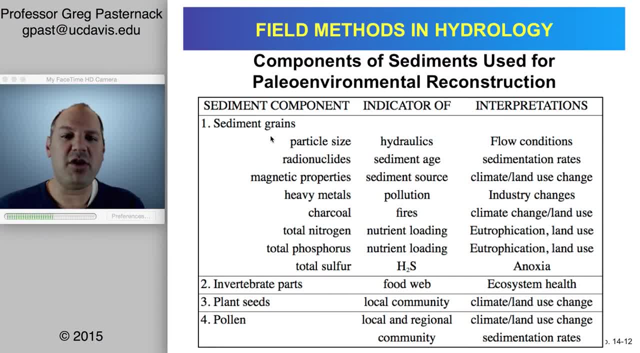 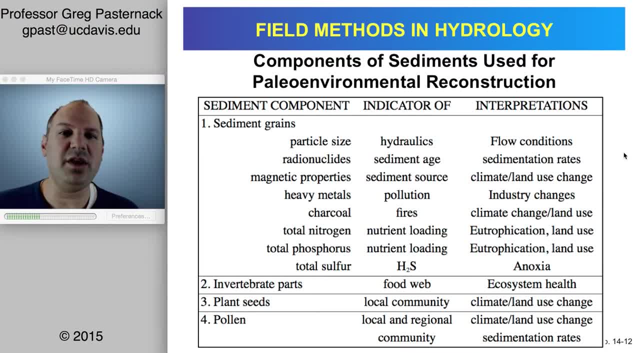 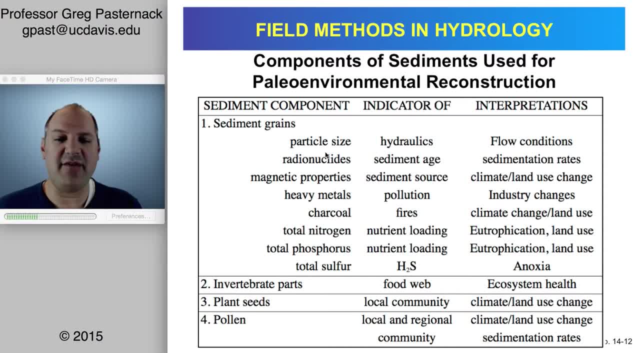 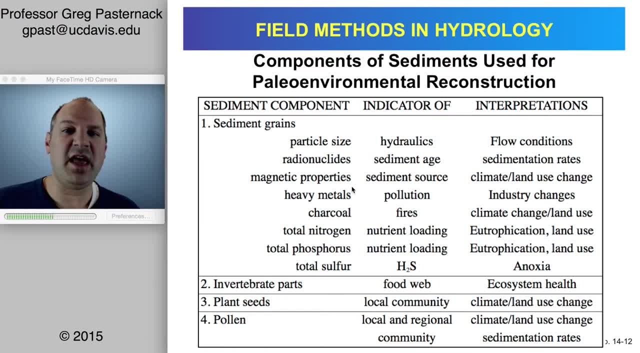 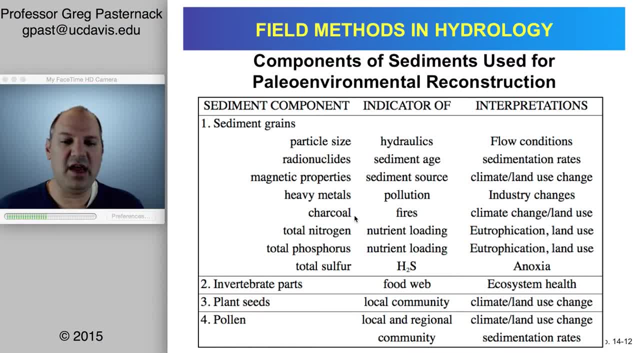 particles or degradation of the particles to indicate the history of fires in a watershed or an airshed, And then other chemicals that may be present related to nutrient cycling and contamination. There are people- I think I mentioned this before- people with forensic kind of skills. 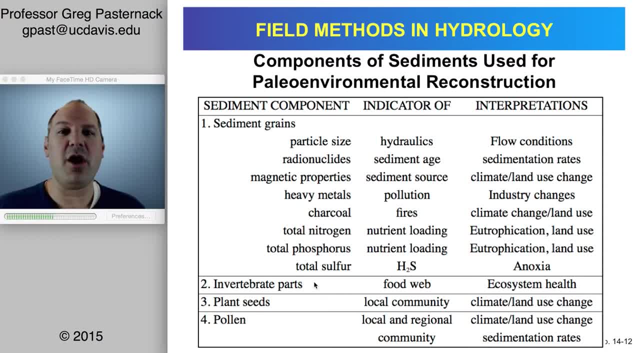 where their expertise is, certain invertebrate parts or pollen, grains or plant seeds and all these biological materials can be really amazing for hydrology to be able to understand the relationship between the water balance and different aspects of ecology, such as food web, the composition and structure of a community. 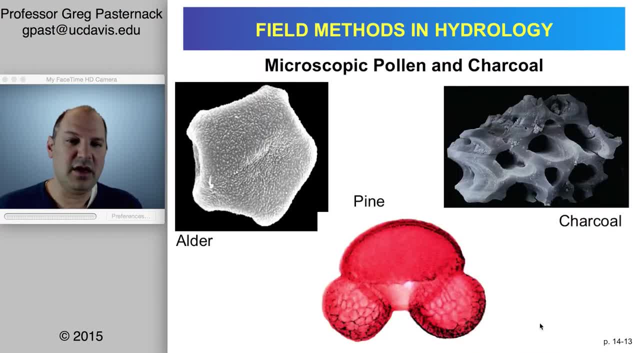 At local level, At local and regional scales. Microscopic particles can include charcoal, but also pollen grains, and here are two examples. So if you take sediment from the bed of a river or in a wetland or at the bottom of a lake and then you can actually dissolve the inorganic material away with inorganic 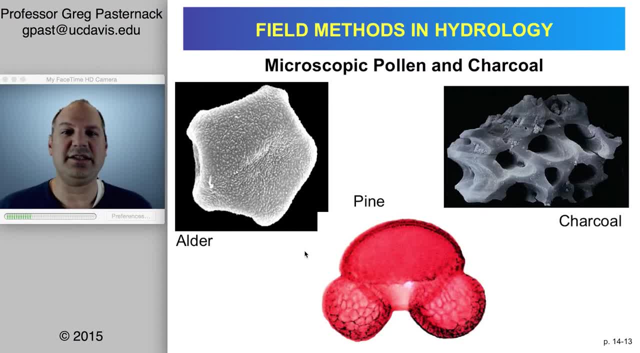 acids like hydrochloric acid, sulfuric acid, nitric acid, and be left behind with the organic materials. Because, remember, from the container for water sampling like affects like, And so you can extract out pollen and charcoal and then analyze them under a microscope to 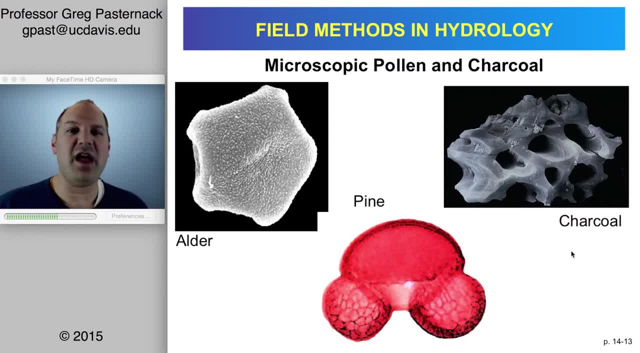 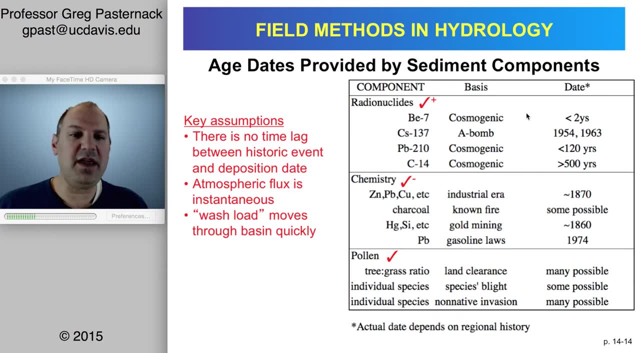 learn a lot about what the composition of the watershed and or airshed was at different periods of time in the past. There are things that we can date and really getting dates is very, very important part of these tracers in the environment. There are things that we can date and really getting dates is very, very important part. 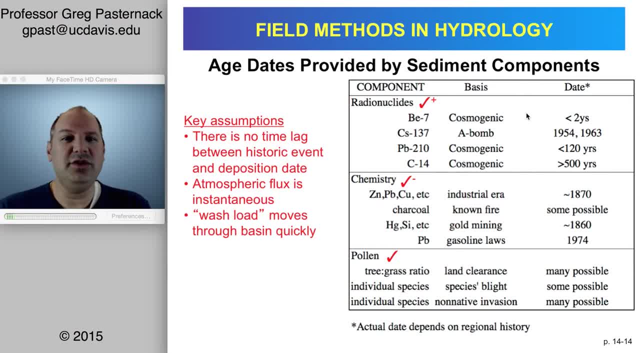 of these tracers in the environment. You know, when you go deeper and deeper into sediment, you're going further back in time. But exactly when is an essential aspect, And so, of course, radionuclides do that. With the radionuclide, you have materials falling out of the atmosphere and depositing 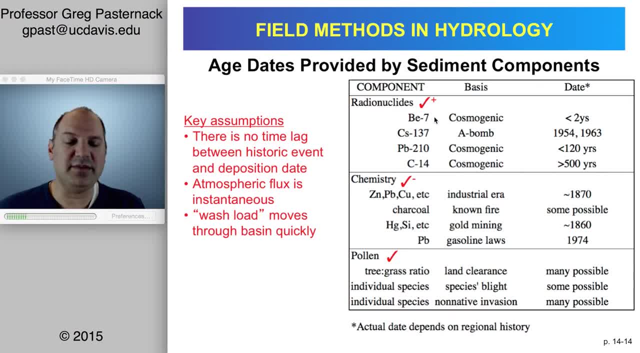 And so that would be like the effects with beryllium-7 in sediment. We have cesium-137 and lead-210 that can accumulate in sediments, And then also we have the radiocarbon dates. These are the ones that are associated with the organic matter that's dead versus living. 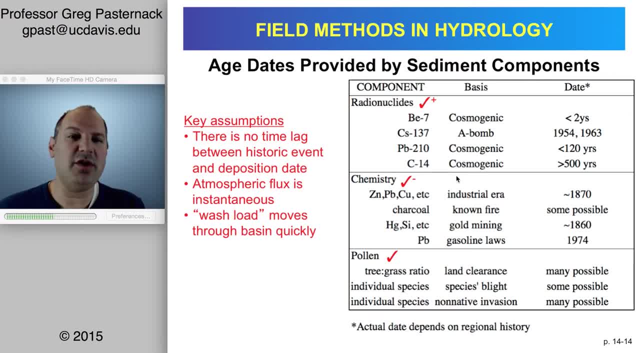 and telling you when it died, And this isn't a course where we're going to go into the mechanisms of radionuclides. That's something that I cover in my Hill Slope Geomorphology and Sediment Budgets class. 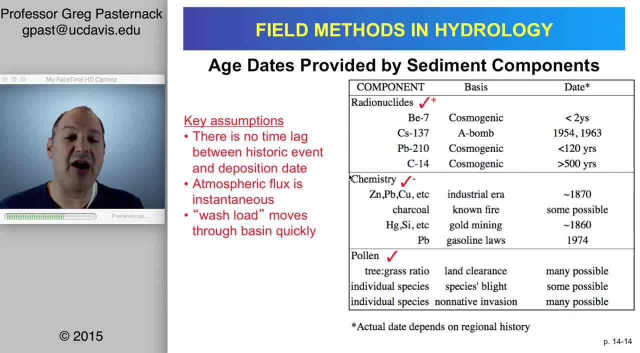 But this just gives you a feel that these are out there And there are courses in isotope geochemistry that you can take if you want to learn more about those. Similarly, for the chemistry, We're not going to go into the details of the reactions and transport of these materials. 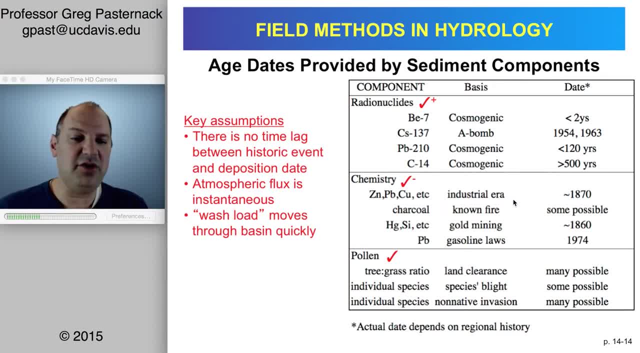 But I just want you to know that these different constituents can tell you things like the onset and progress of the industrial area with heavy metals or, in California, where we have gold mining, mercury and silica concentrations, tell you about the passage of the hydraulic mining sediment that's present. 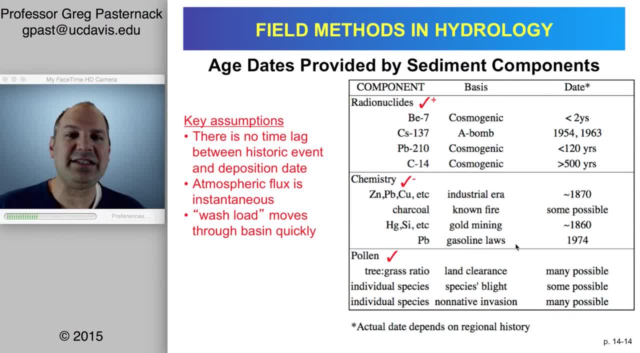 And then in lots of areas when leaded gasoline was phased out. in the United States it was phased out in 1974. And so you see an abrupt change in the abundance of lead in the environment after that. We can also learn about the age of things by comparing things that we see in the historical. 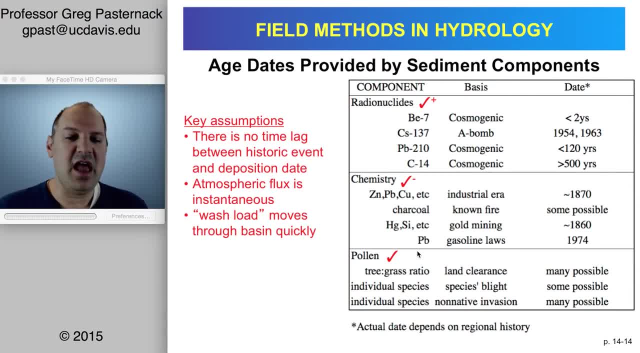 record, the written record of our society against things that take place in the environment. So, for example, we know that with European colonization of the east coast of the United States there was a lot of land clearance that took place. And we can see in the environment that there was a lot of land clearance that took place. 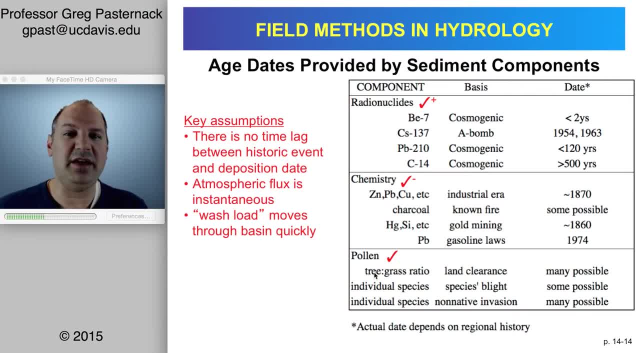 And we can see in the environment that there was a lot of land clearance that took place And we can see in the environmental record a transition from tree pollen to grass pollen. So we just have to look for when those transitions are found in sediment and line that up with. 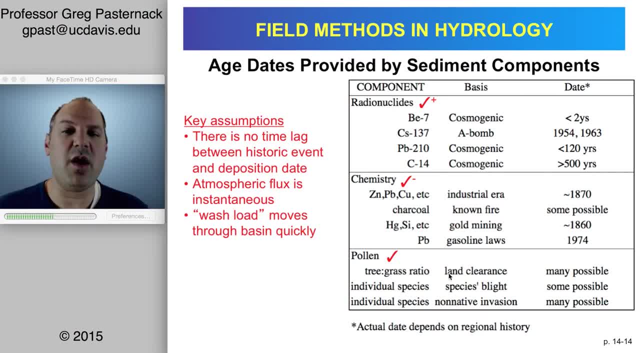 the historical records of when land clearance took out in a watershed, And then we can get a date based on that. Similarly, you might have a species of plant that either was introduced like an invasive or was lost through some sort of disease or deforestation or something. 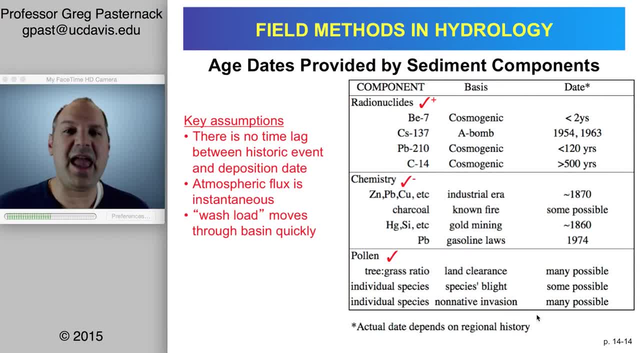 And so those can be used again comparing against historical records to get dates. And these are all important to be mindful of because you know, sediment can be a very powerful tracer for understanding the hydrology of a watershed. And these are the constituents of sediment. 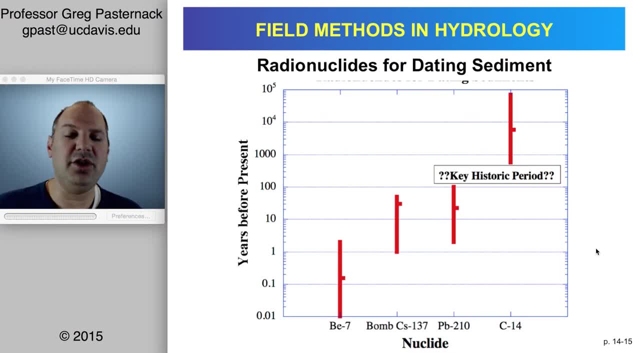 One of the things that's challenging about using tracers: when you're not tracing over, you know mere rocks across the coast. I know they're all really way too disconnected. Certainly you know you could use multiple 지난ites of sediment long after you somehow. 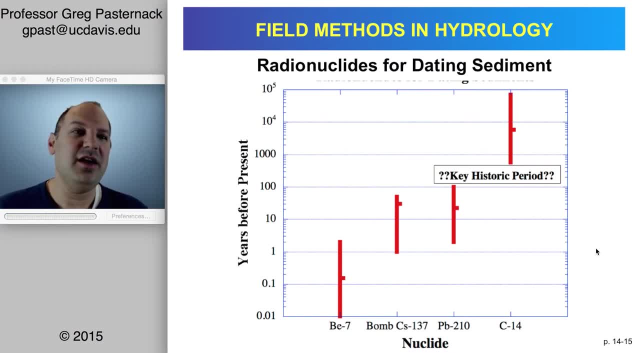 know minutes to hours, to days, like with- uh, you know a release of a dye in a river or something like that, but when you're really wanting to trace over years, to say 100 years or 200 years, like basically to understand the effects of, you know, modern european expansionism around the world. 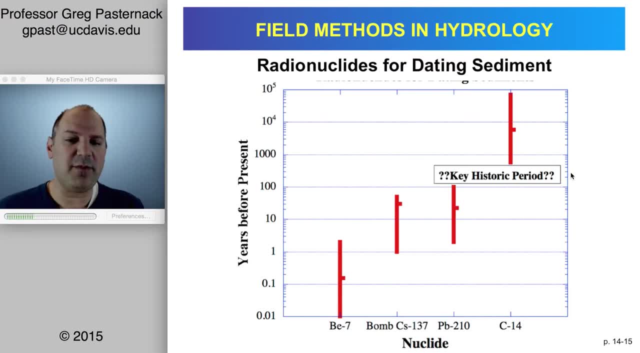 then, when you get into that key historic period of 100 to 500 years ago, unfortunately we hit a gap where there really aren't a lot of good dating methods that work led to 10 is a method that goes back typically 120 years, and then radiocarbon dating tends to, you know, be like you know. 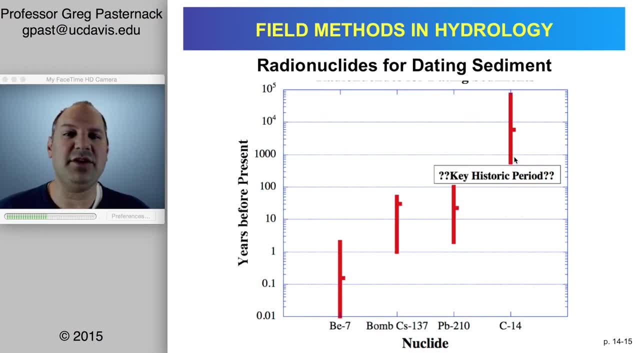 thousands of years down to, you know, 500 plus years. now there are some ways to use radiocarbon dating that can get more recent to that, and it just depends on the nature of the materials you have in the situation and the the type of dating that you. 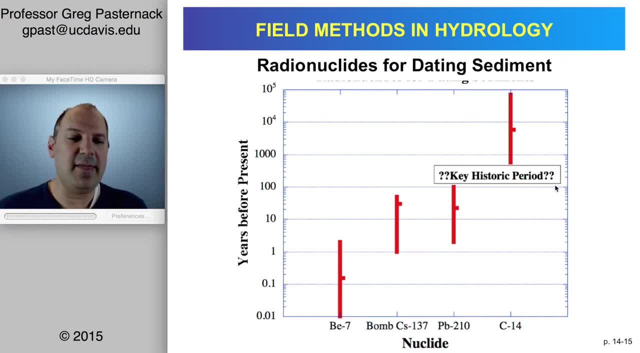 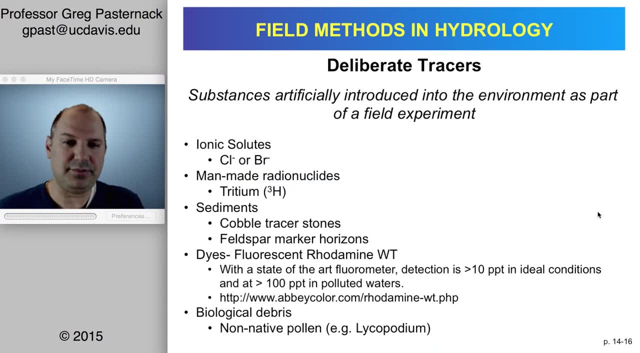 use, but it is generally tough to get environmental tracing information from this key historic period of european colonization around the world. Okay, deliberate tracers: these are substances artificially introduced to the environment as part of a field experiment. I wish we could do tracing a lot more. 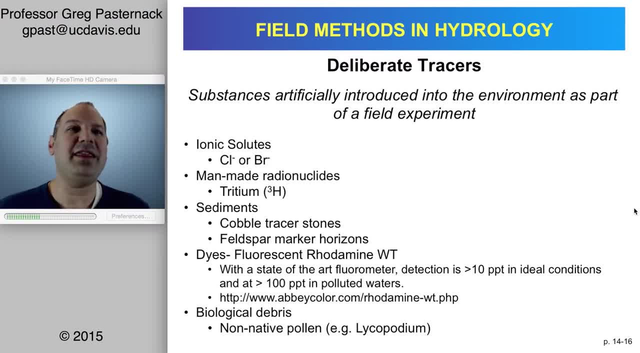 but the reality is that people don't like the idea of scientists going out and polluting, basically, and of course, pollution has become so ubiquitous in the environment that any tracing that we do would likely have a really small to negligible impact. but you could see the example in: 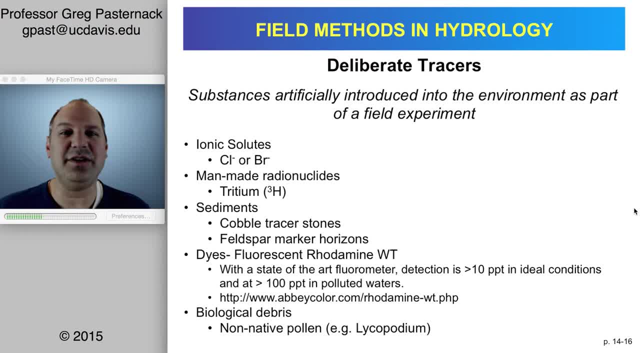 oceanography. you know, we can't be going out throwing 60,000 buoys and tracers. if, if you know, if we're going to have boating accidents that are going to release those, we should. we have to be opportunistic and take advantage of that. but it's just, society sort of draws a line, there's only so. 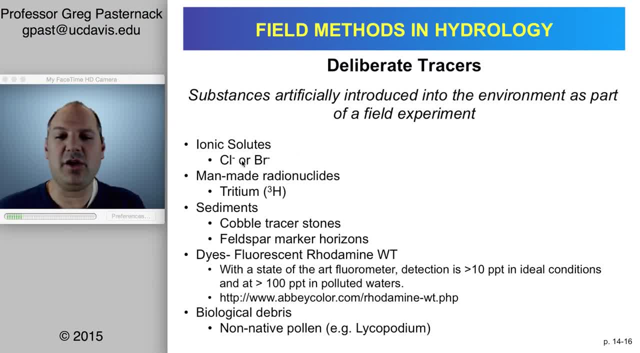 much that we can do to make sure that we're not just throwing 60,000 buoys and tracers. but we're we can do, and some things are easier, like chloride or bromide. you know, dissolution is relatively simple thing with relatively low consequences, where, in contrast, a man-made nucleoid like tritium 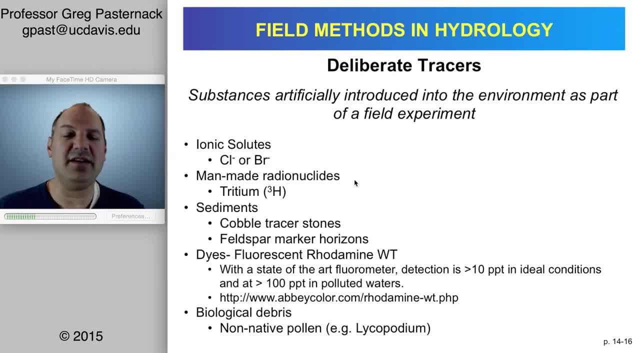 has to be obtained from a radioactive source and then you're introducing that radioactivity into the environment. so, although this is a very useful tracer, it's something that is very rarely used anymore. Sediments: these are used for a number of reasons. these are used very extensively. we had the cobble tracer stones I showed in the 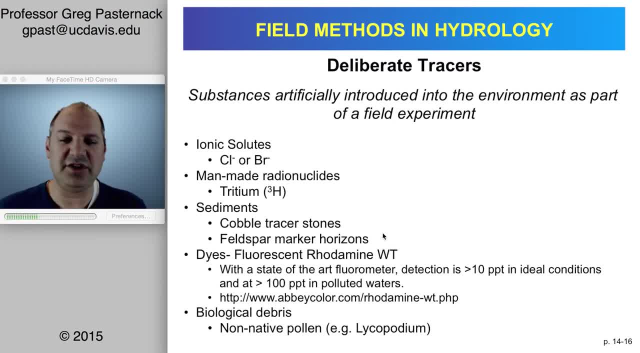 very first the cover page of this presentation. when we talked about surface sediment erosion deposition rates, I showed the Feldspar marker horizon. well, that's, that's a tracer. the most common one are dyes for looking at, you know, free water flows, then we can inject dyes in the appropriate. 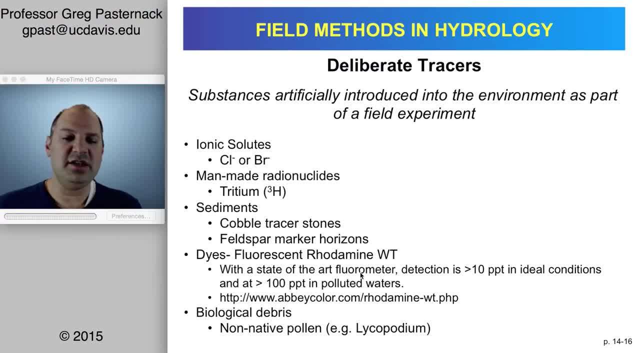 concentration and use something called a fluorometer to detect the concentration at down gradient locations, and fluorescent rhodamine, WT, is the most commonly used one, but there are a variety of different dyes for different circumstances and I've given you a website, you know link here that you can. 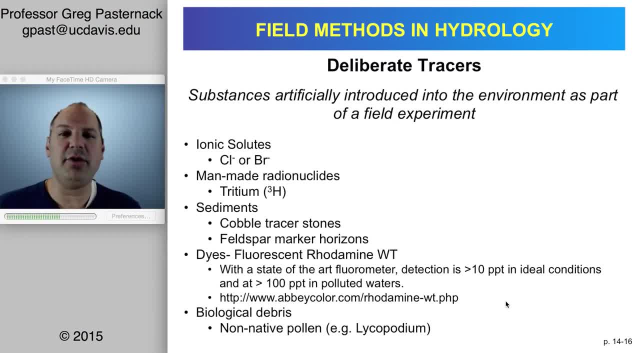 use to learn more about that. we actually do have the capability to do this kind of tracing in in my department, and it can be really useful for getting discharge and estimating parameters necessary for different models. and then, finally, sometimes we do introduce biological debris that isn't native to that area of 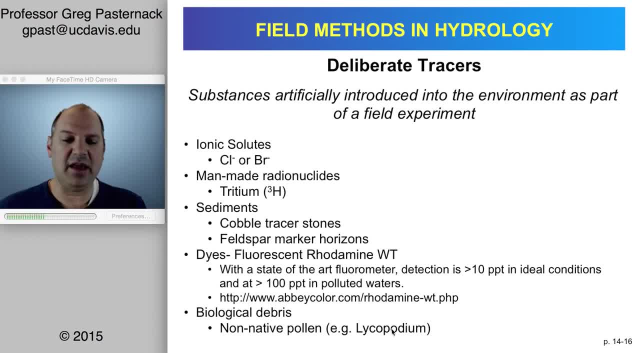 study, and one of those is non-native pollen. there's a type called like a podium. we use it more in a laboratory setting and then an environmental setting, but we use it to dope samples so that we can have a count and and get a get something that is independent of what the naturally 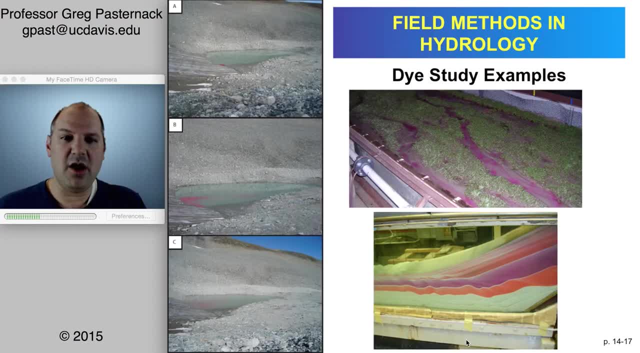 occurring pollen is OK. then here's just a few examples of dye study. in the left is a small lake. you can see that the die introduced in the lower left of the lake and then it spreads around through time. you can see the large, concentrated but relatively small areas and then, much later, the diffuse. 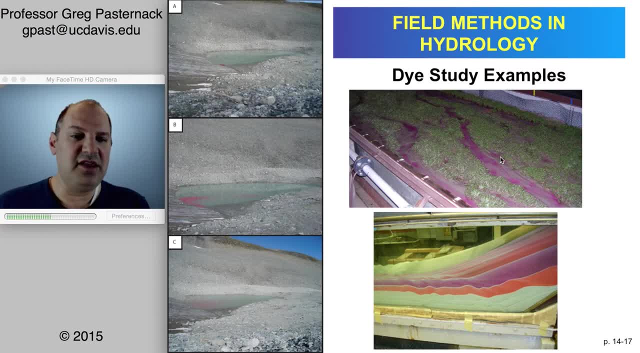 low concentrations more ubiquitously. looking at in the upper right when a die is being used, in this case, where we have a flume experiment studying sediment transport dominated by bed load- but to look at the role of vegetation that would be occurring in a large river here to give you a sense of scale. this 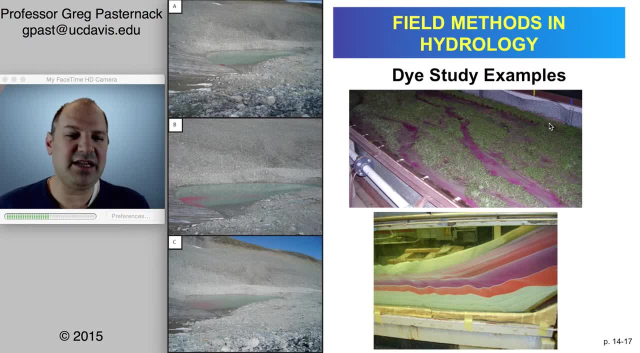 this width here. i would say it's somewhere between like five and ten meters wide, from my memory, and maybe you know 30 meters or 40 meters long, something like that. and here what you can see, the dye like the darker pink is occurring where the water is deeper and the lighter pink where 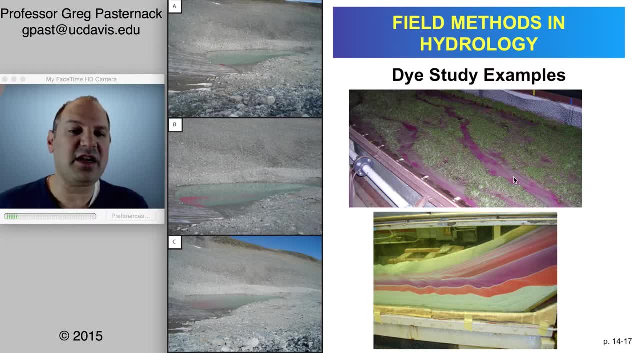 it's shallower. so, based on this color, you can just take a photo from above and be able to see the concentrate or the water depth based on the concentration. so here the tracer is being used to help reconstruct the topography of the land as it's changed by the flow, and then in this bottom, 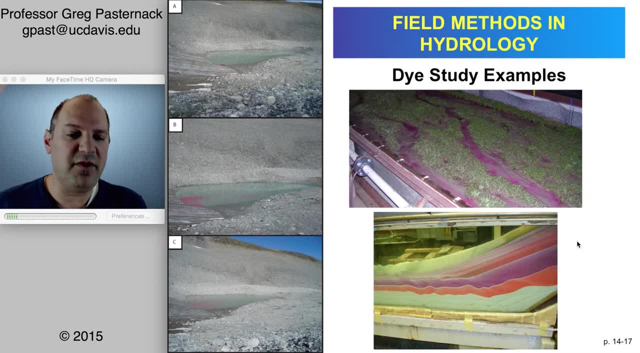 example, this would be a continental shelf flume experiment where different colors are used to show different epochs of deposition and you can see how that sediment is being dispersed down out into the deeper parts of the ocean in this kind of flume experiment. so you know, traditionally you probably didn't think about. 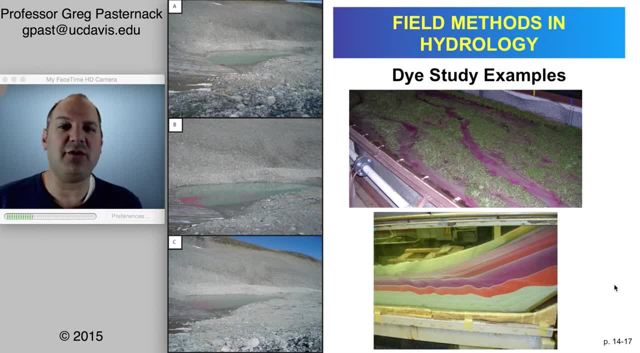 tracers as a topic that we might cover in a field methods and hydrology class. but in fact there's a huge link between field methods and tracing and you know a lot of field studies. if there's an opportunity to do that, you can do that in a field methods and hydrology class and you can do that.